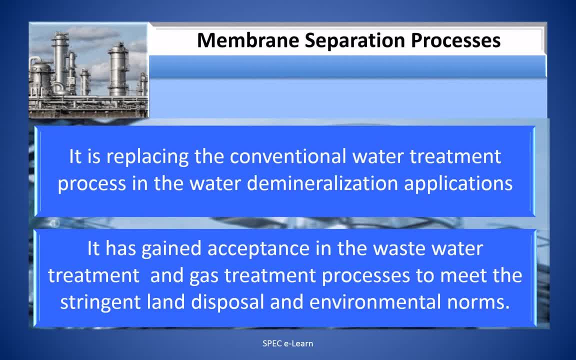 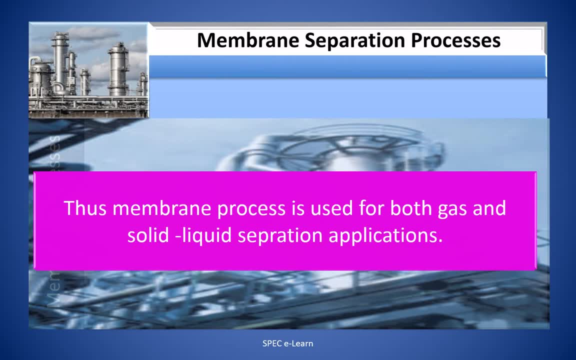 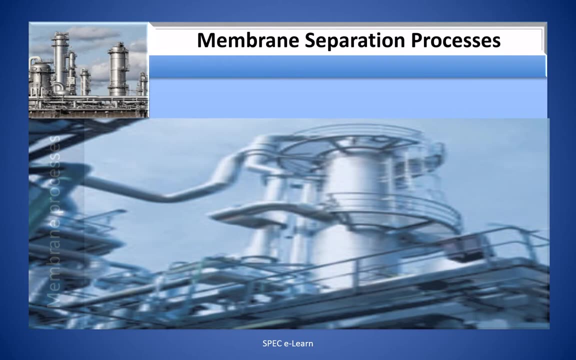 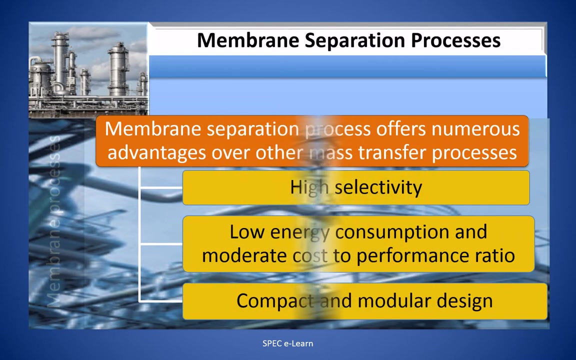 to meet the stringent land disposal and environmental norms. Thus, the membrane process is used for both gas and solid liquid separation applications. Membrane separation process offers numerous advantages over other mass transfer processes: 1. High selectivity, 2. Low energy consumption and moderate cost-to-performance ratio. 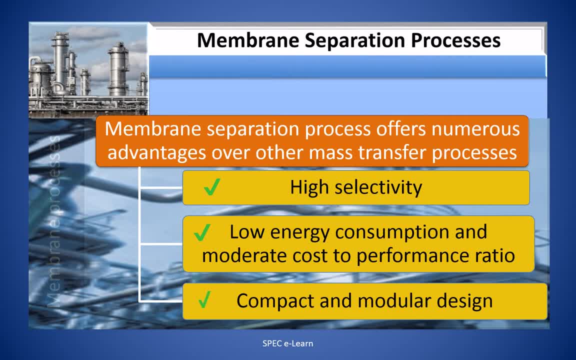 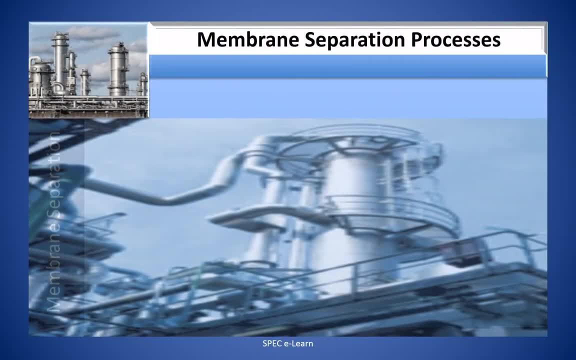 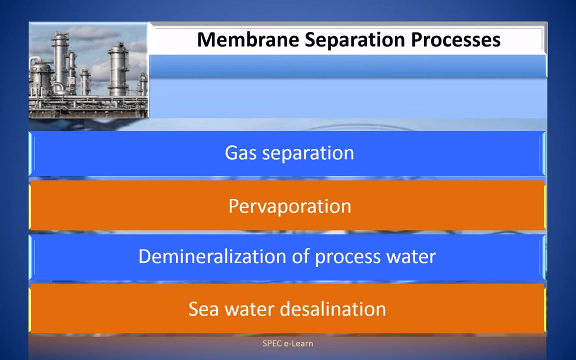 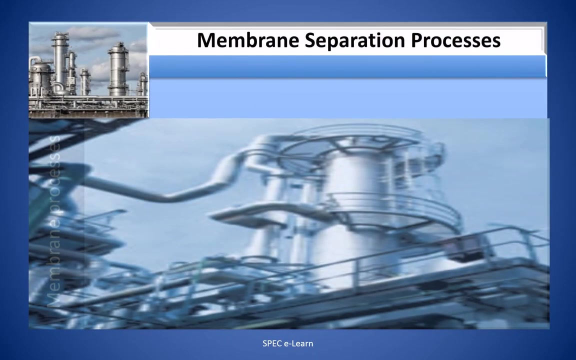 3. Compact and modular design. Membrane separation process offers numerous advantages over other mass transfer processes. Typical applications of membrane process include gas separation, pervaporation, demineralization of process water and seawater desalination. What is Membrane separation process? 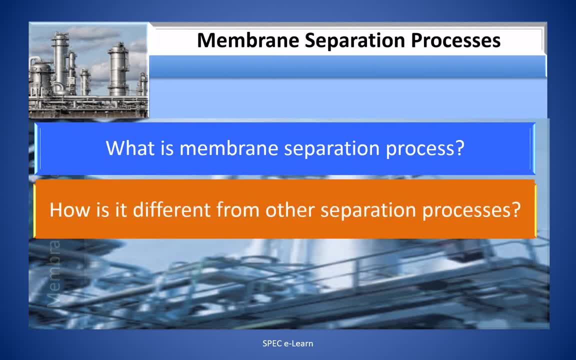 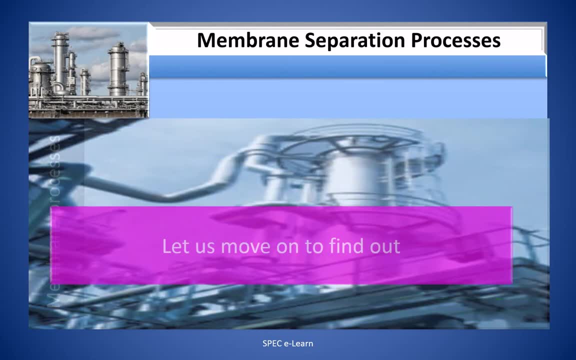 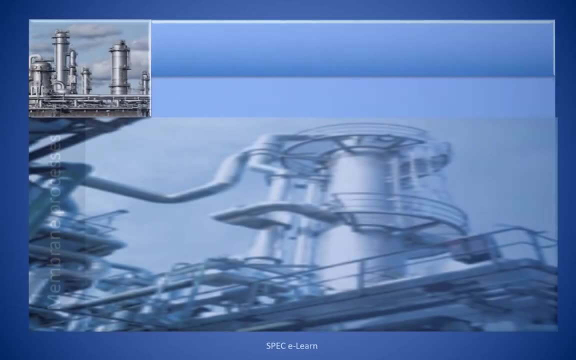 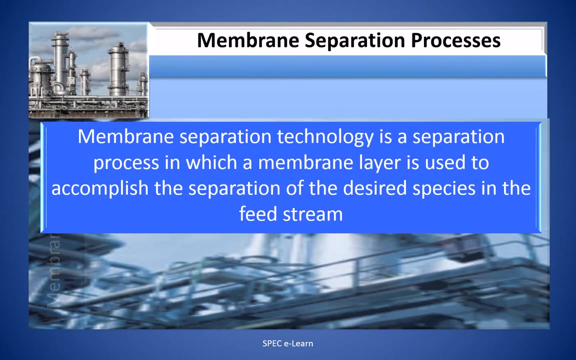 How is it different from other separation processes? What factors are working in its favor and contributing to its acceptance by the industry? Come on, let us move on to find out. Membrane separation technology is a separation process in which a membrane layer is used. 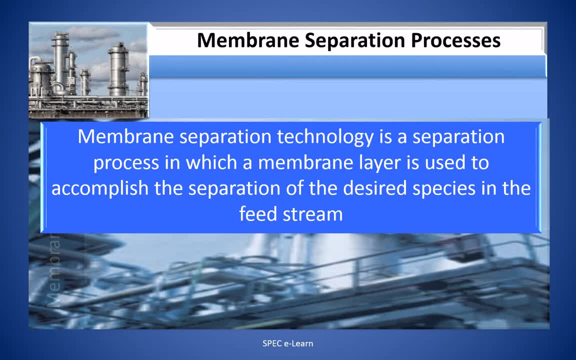 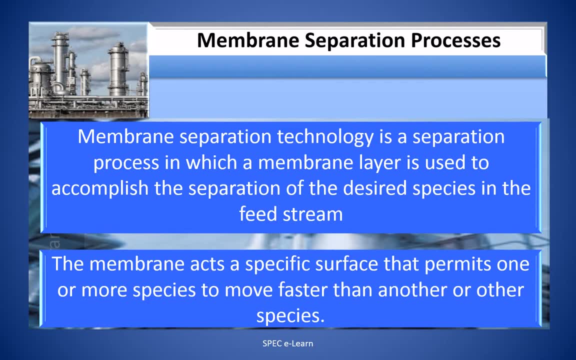 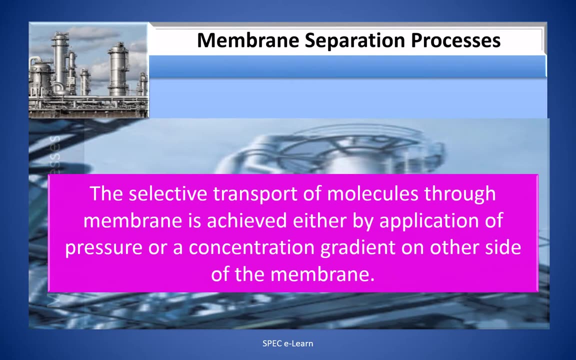 to accomplish the separation of the desired species in the feed stream. The membrane acts as a specific layer. The membrane acts as a specific surface that permits one or more species to move faster than another or other species. The selective transport of molecule through the membrane is achieved either by application of pressure or a concentration gradient on the other side of the membrane. 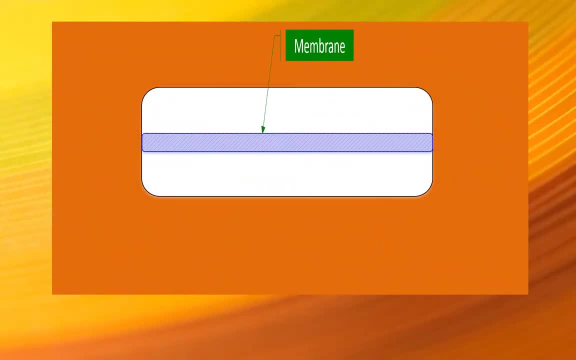 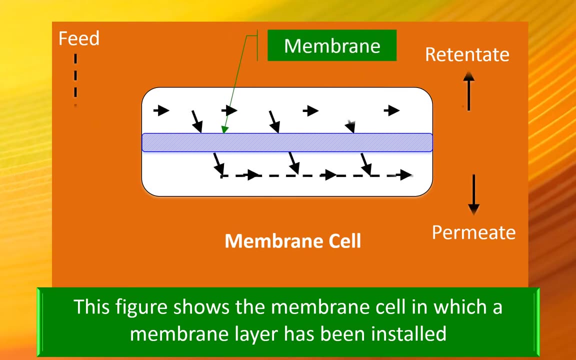 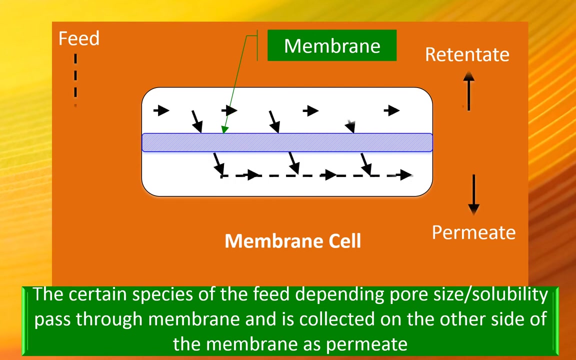 This figure shows the membrane cell in which a membrane layer has been installed. The feed enters at the top and flows through the cell over the membrane surface. Certain species of the feed, depending on the pore size or solubility, pass through the membrane and is collected on the other side of the membrane as permeate. 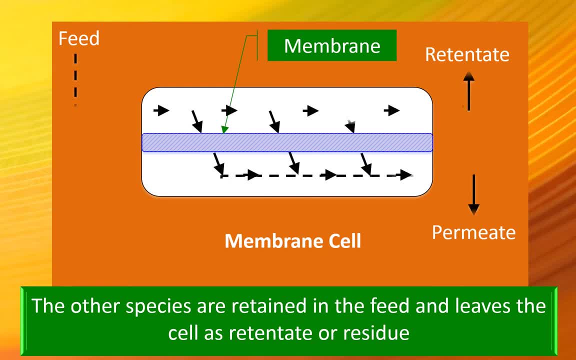 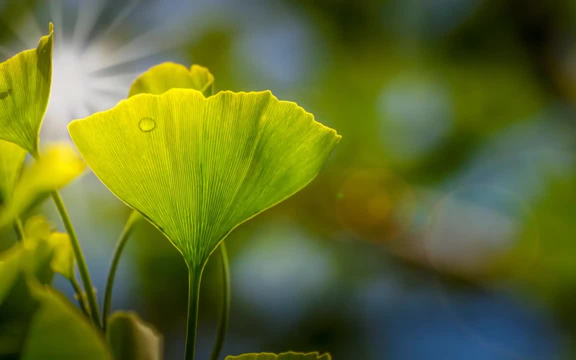 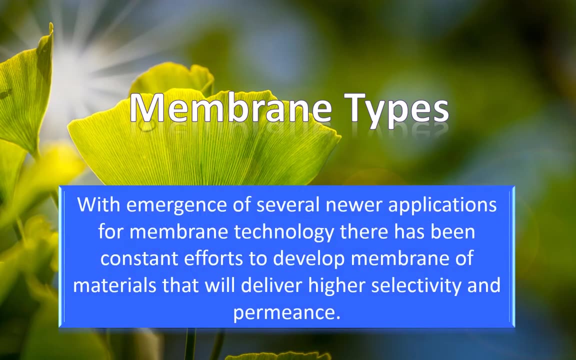 Other species are retained in the feed and leaves the cell as a retentate or residue. Membrane types. With the emergence of several newer applications for membrane technology, there has been constant efforts to develop membranes of materials that will deliver high selectivity and permeance. 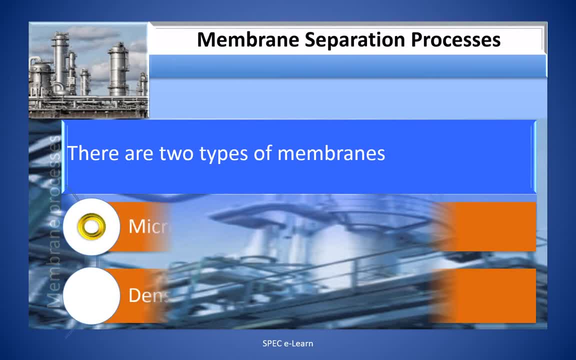 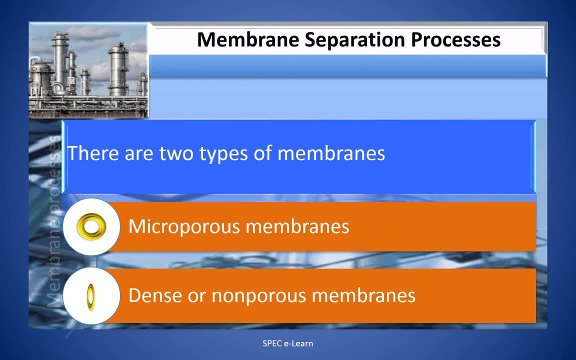 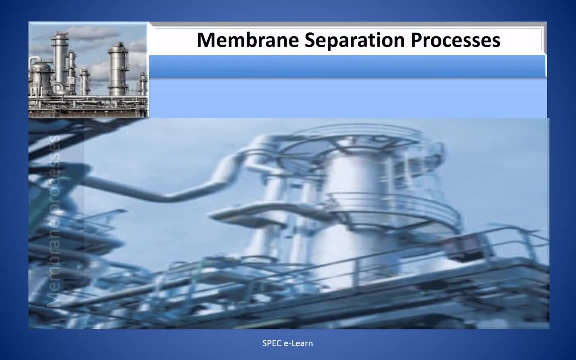 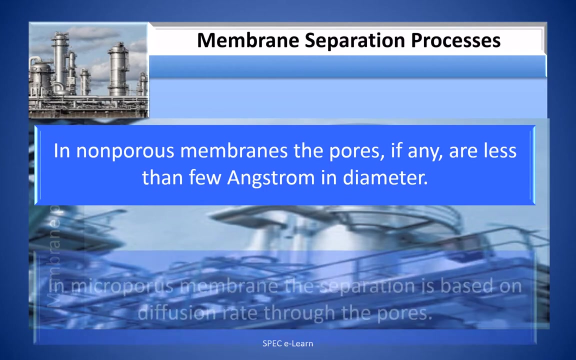 There are two types of membranes, One microporous membranes, Two dense or non-porous membranes. jak erstmal First the determination of the In non-porous membranes, the pore, if any, is less than the few angstroms in diameter. 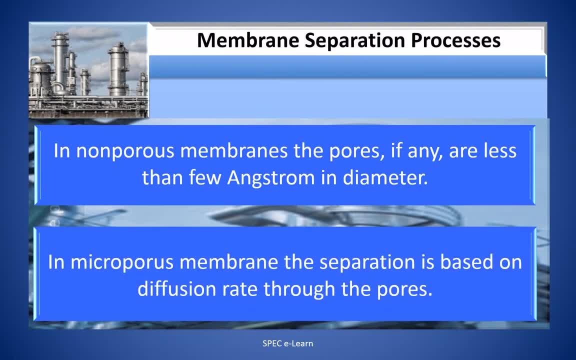 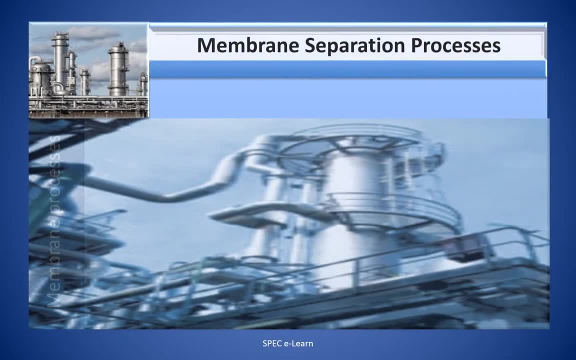 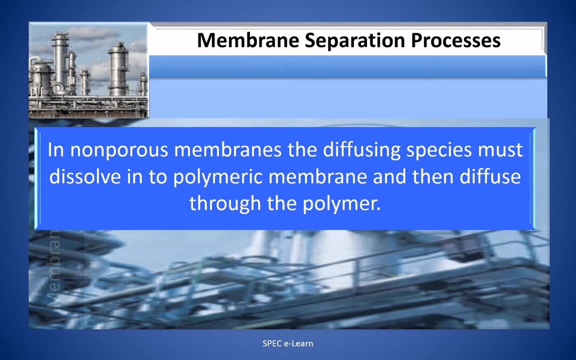 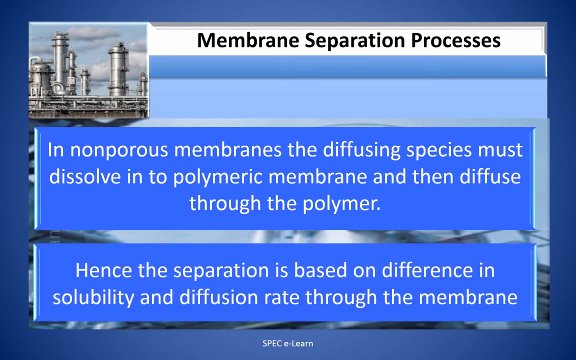 In microporous membranes, the separation is based on defined rate through the pore Skines, Serum Acid Filtration. In non-porous membranes, the diffusing species must dissolve into the polymeric membrane and then diffuse through the polymer. Hence the separation is based on difference in solubility and diffusion rate through the 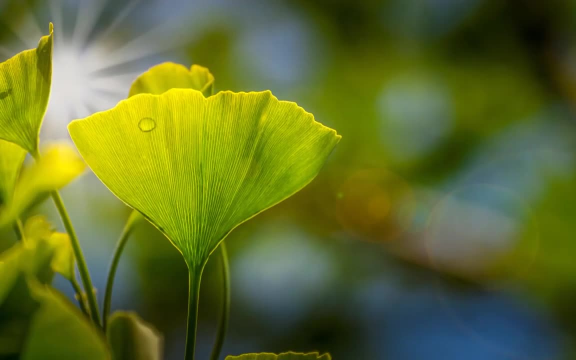 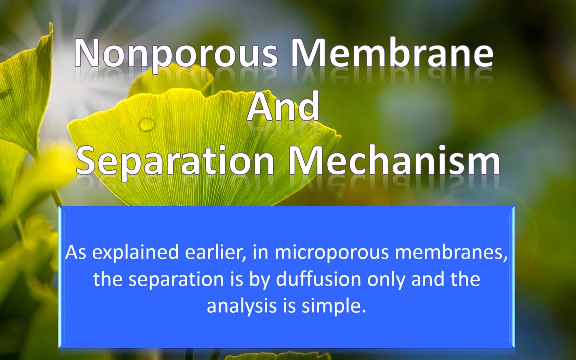 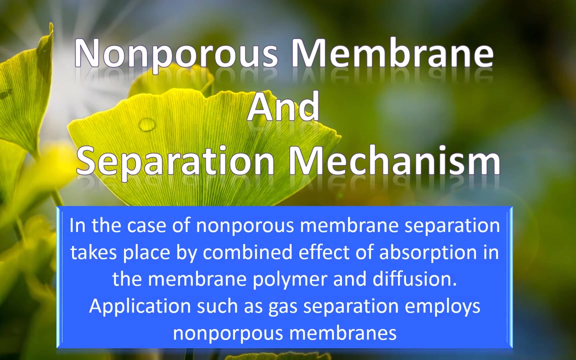 membrane, Non-porous membrane and separation mechanism. As explained earlier, in microporous membranes, the separation is by the diffusion only and the analysis is simple. In the case of non-porous or dense membrane, separation takes place by combined effect of absorption in the polymer and diffusion. 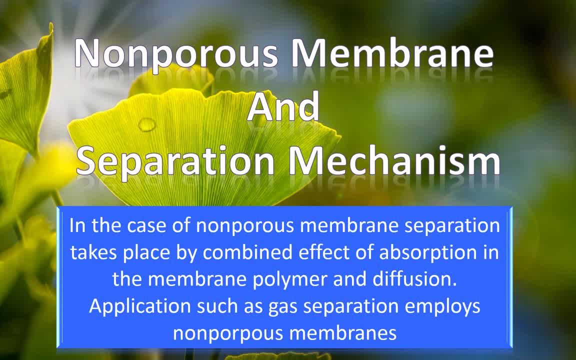 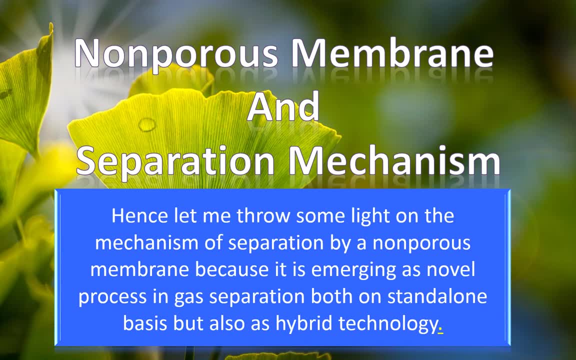 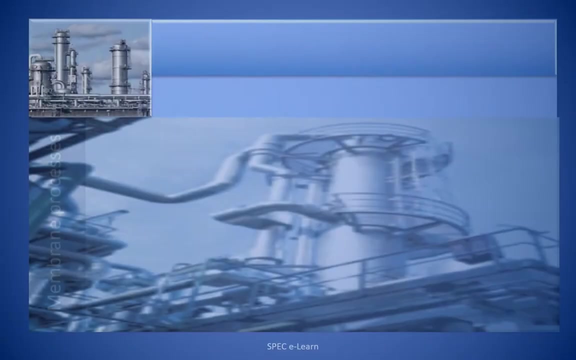 Applications such as gas separation employs non-porous membranes. Hence, let me now throw some light on the mechanism of separation by a non-porous membrane, because it is emerging as a novel problem- The process in gas separation, both on standalone basis, but also as a hybrid technology. 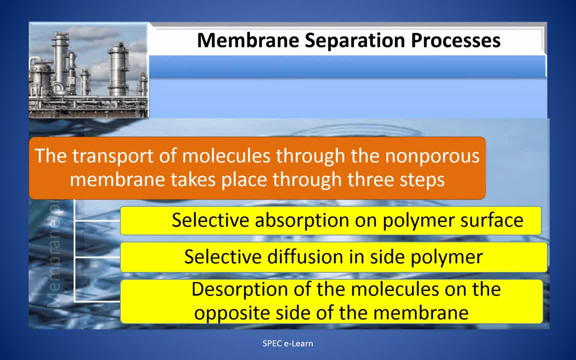 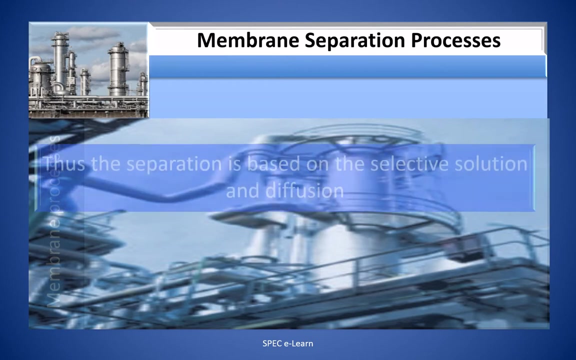 The transport of molecules through the non-porous membrane takes place through three steps: Selective absorption on polymer surface, Selective diffusion inside polymer Disorption of the molecules, Selection of the small particles and곳ige ciudad not dependent, And then on the opposite side of the membrane. Thus the separation in a non-porous membrane. 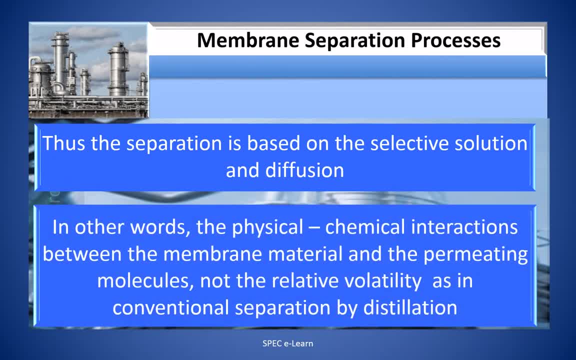 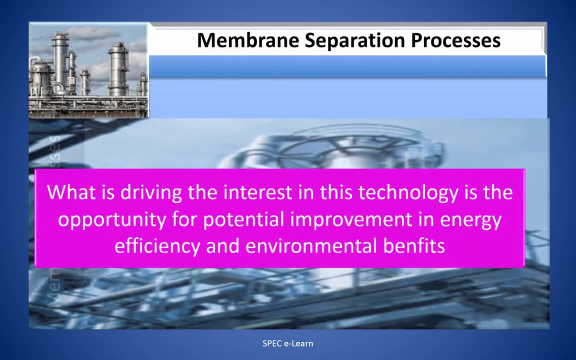 is based on the selective solution and diffusion, In other words, physical chemical interactions between the membrane material and periminating molecules, and not the relative volatility as seen on conventional separation by destellation. What is driving the interest in this technology is opportunity for potential improvement in energy efficiency and environmental benefits. 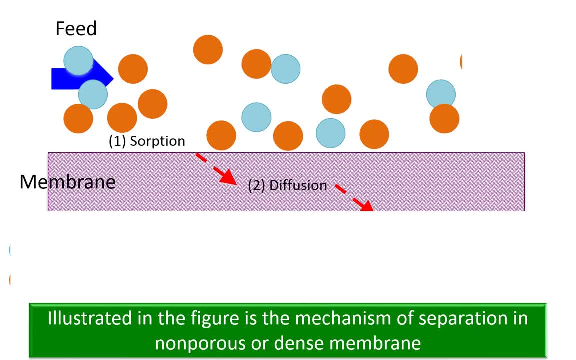 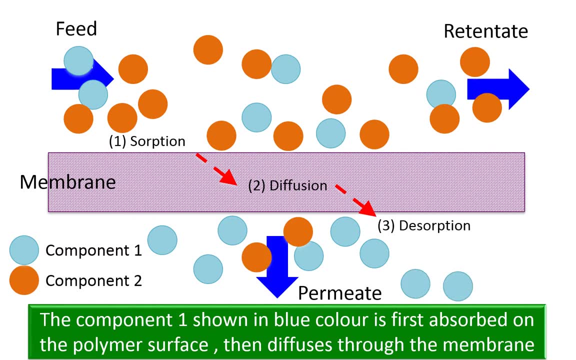 Illustrated in this figure is a mechanism of separation in a non-porous or dense membrane. The component 1, shown in blue color, is first absorbed on the polymer surface, then diffuses through the membrane, finally gets desorbed from the surface of the membrane on the accessory of the membrane. 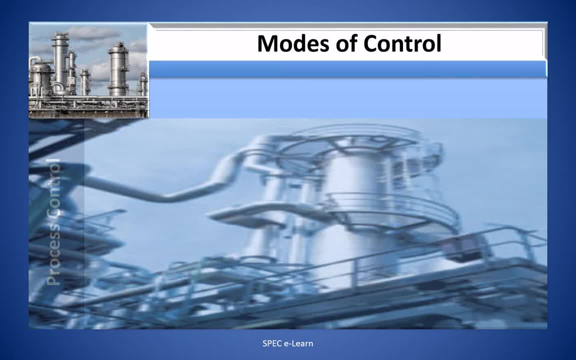 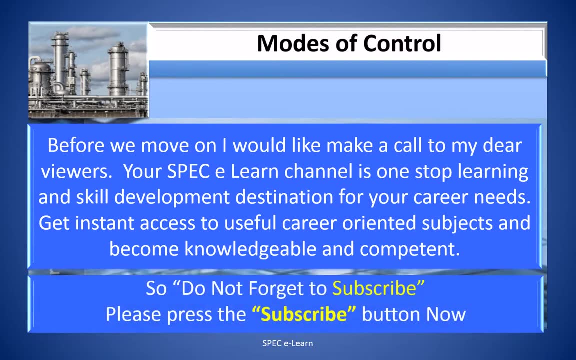 Before we move on, I would like to make a call to my dear viewers. Your SPEC eLearn channel is one-stop learning. Get instant access to useful carrier-oriented subjects and become knowledgeable and competent. So do not forget to subscribe. Please press the subscribe button now. 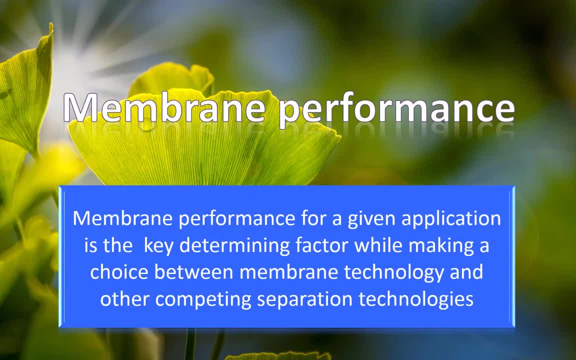 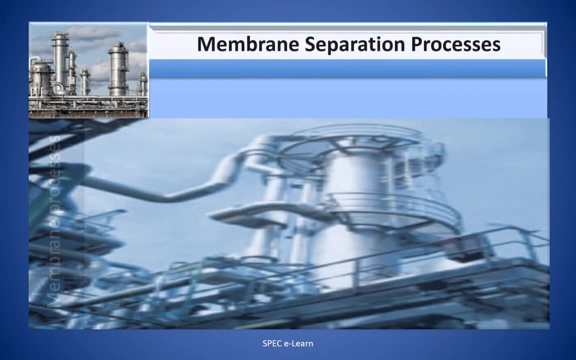 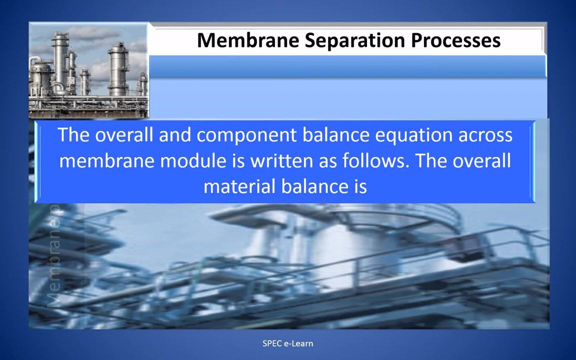 Membrane performance. Membrane performance for a given application is the key determining factor. while making a charge, There is a choice between membrane technology and other competing technologies. The overall and component balance equation across a membrane module is written as follows: The overall material balance is: F is equal to R plus P. 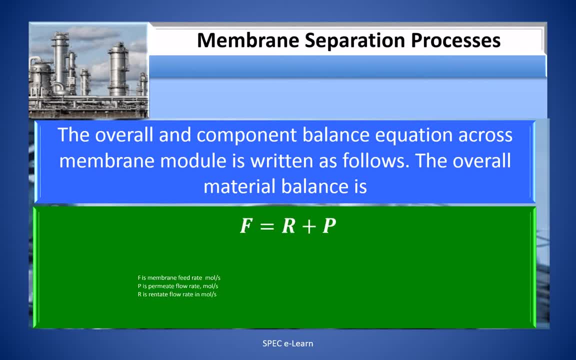 where F is the membrane feed rate in moles per second. P is the permeate flow rate in moles per second. R is the return rate flow rate in moles per second. R is the return rate flow rate in moles per second. 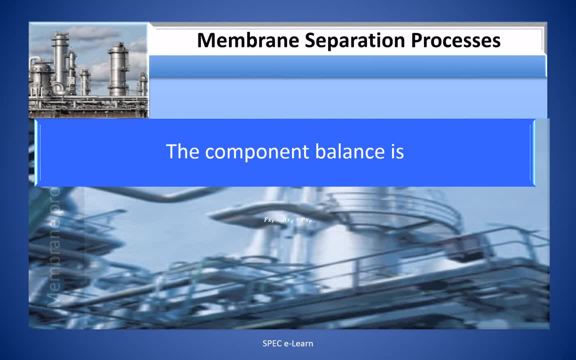 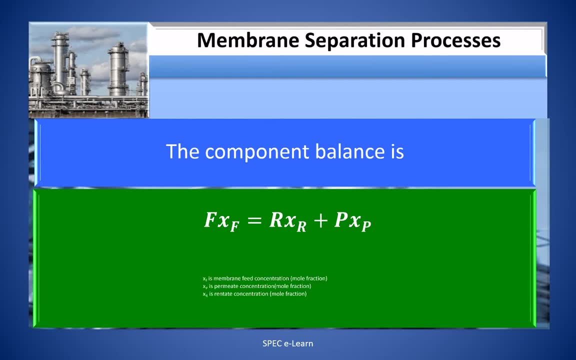 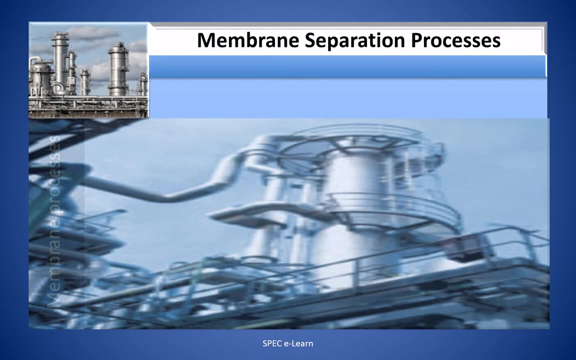 The component balance is written as follows: F times XF is equal to R times XR plus P times XB, where XF is the membrane feed concentration, XB is the permeate concentration, XR is the return rate concentration. The performance of the membrane is characterized by two parameters. 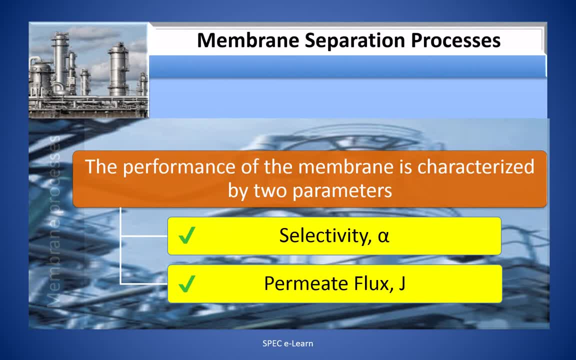 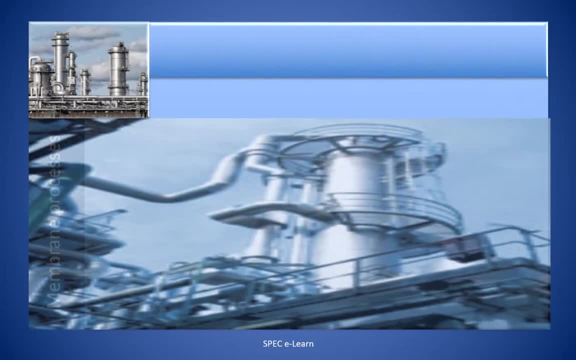 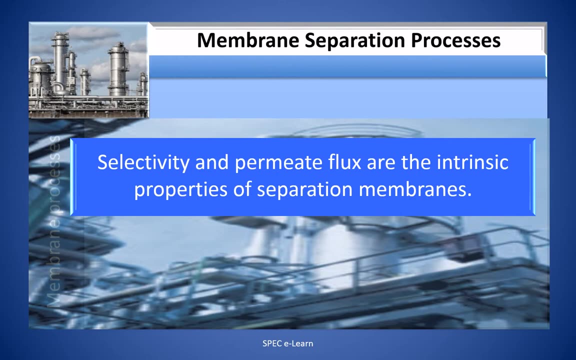 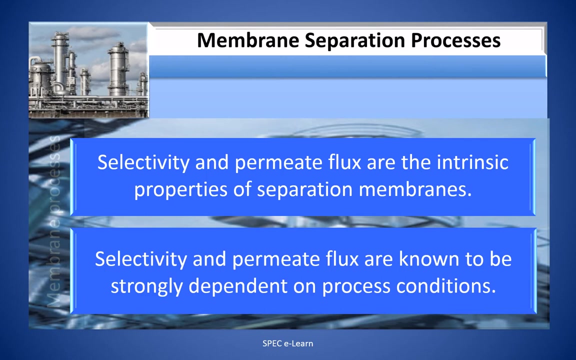 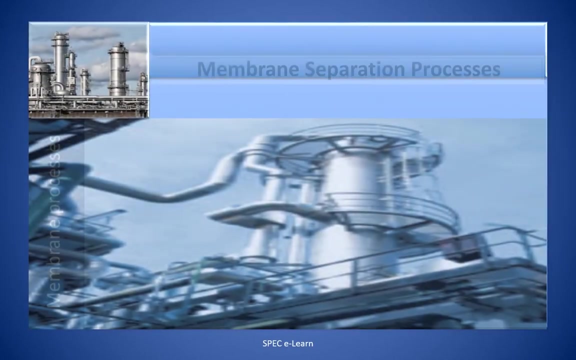 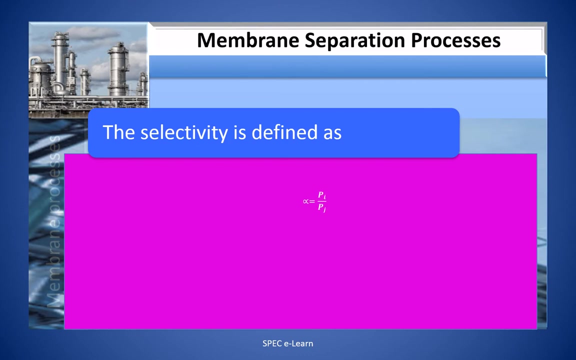 1. Selectivity alpha, 2. Permeate flux J. Selectivity and permeate flux are the intrinsic properties of separation membrane. Selectivity and permeate flux are known to be strongly dependent on process conditions. The selectivity alpha is defined as the ratio of the permeability of component I to the permeability of component J. 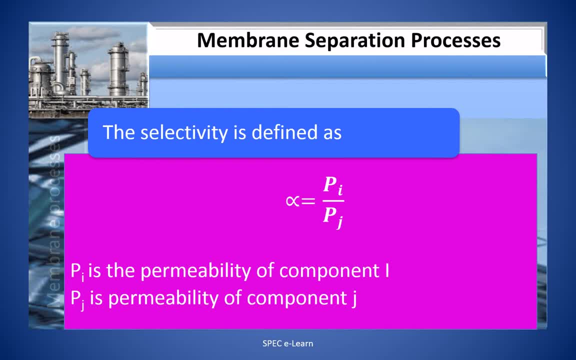 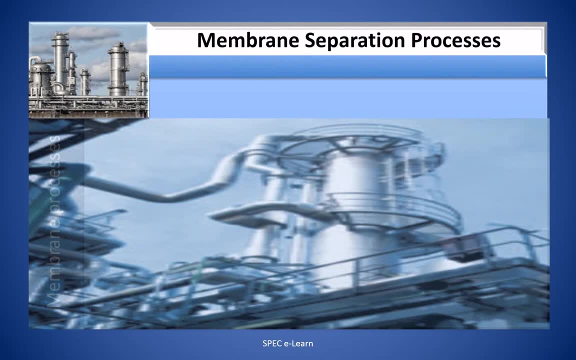 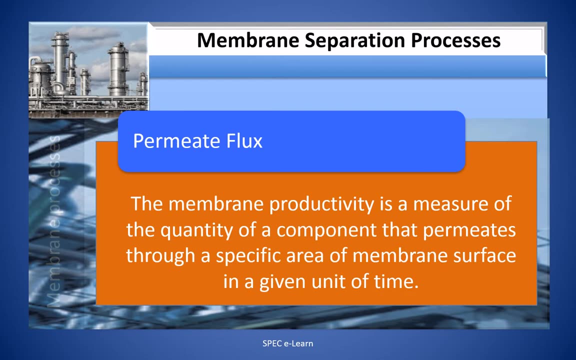 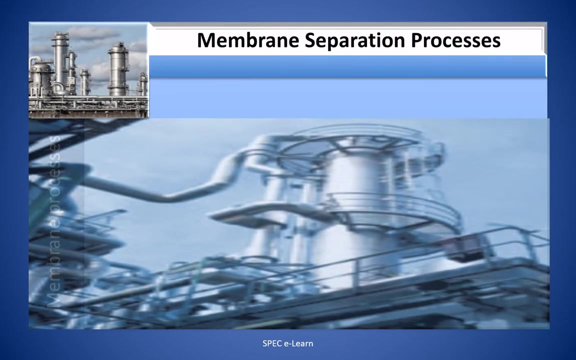 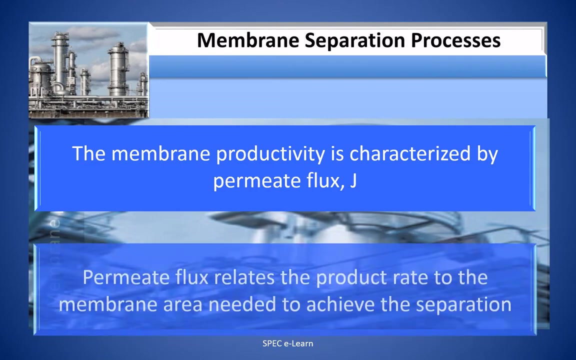 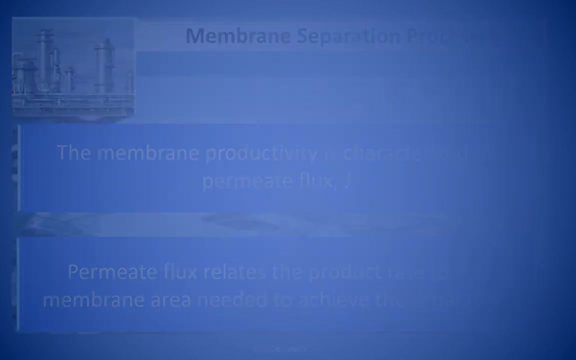 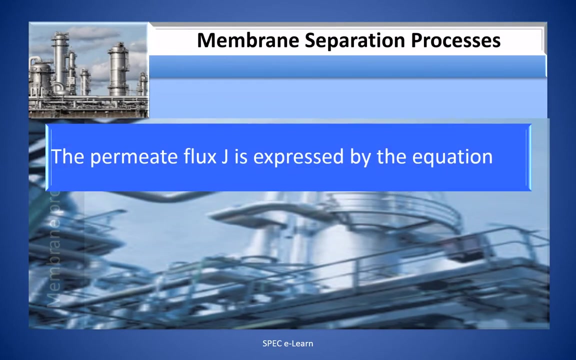 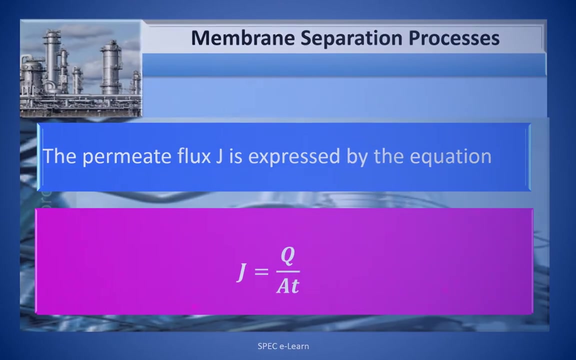 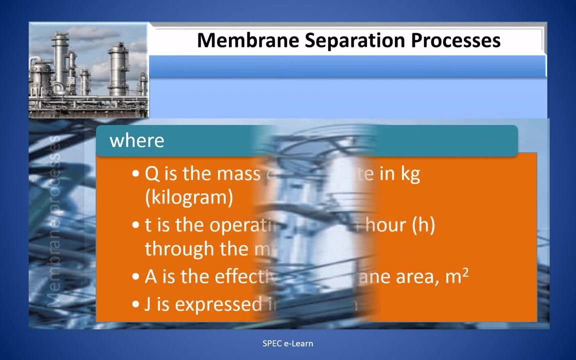 ie PI divided by PJ. Those are the основ two parameters. 2. Permeate flux: The membrane productivity is characterized by premier flux J. Premier flux relates the product rate to the membrane area needed to achieve the separation. The premier flux J is expressed by the equation: J equals Q by AT, where Q is the mass of permeate. 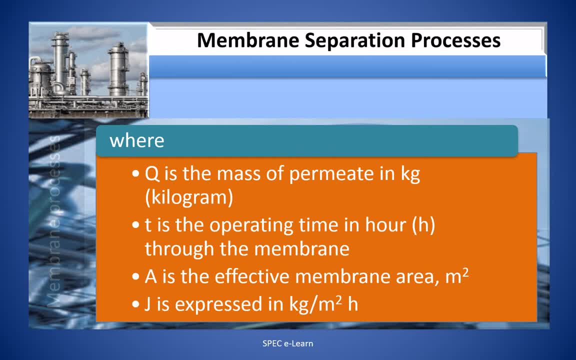 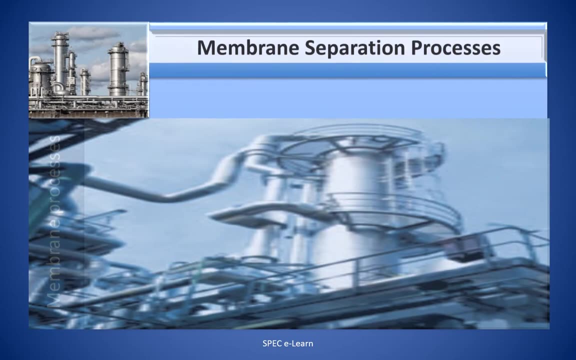 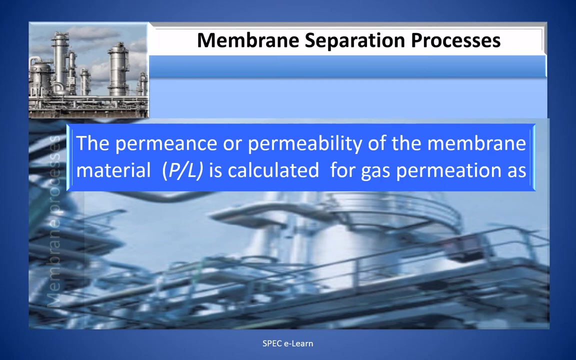 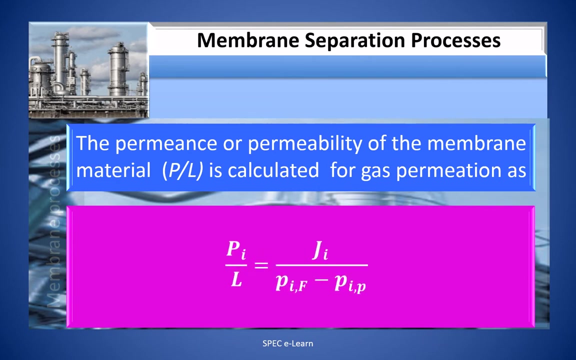 in kg. T is the operating time through the membrane in hours. A is the effective membrane area in square meter. J is expressed in kg per meter squared per hour. The permeance or permeability of the membrane material is calculated as PI by L equals JI divided by PIF. 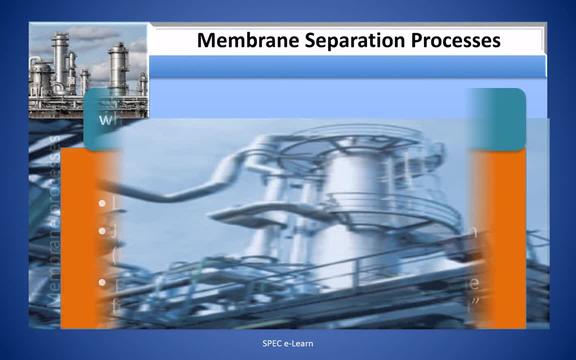 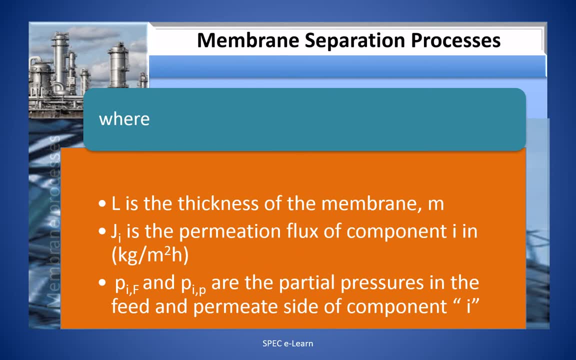 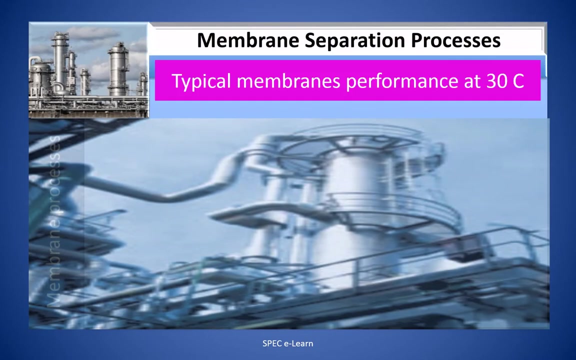 南 اب od 와. membrane in meter Ji is a permeation flux of component I in kg per m2 per hour. Pif and Pip are the posture pressures in the feed and permeate side of the component I. Shown in the table below are the values of permeance and selectivity for separation of: 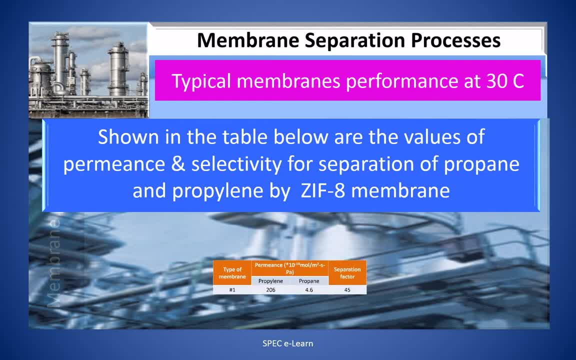 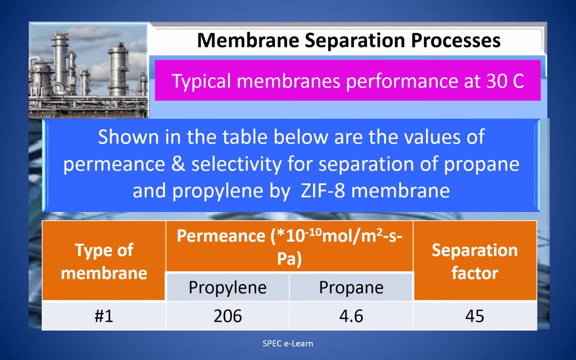 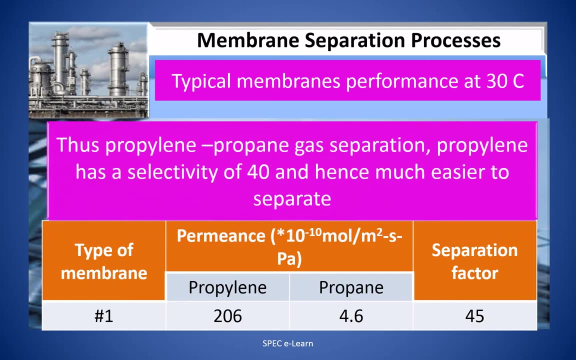 propane and propylene by ZiF8 membrane. The values of permeance of propylene in the units given are 2.06 and that of propane is 4.6.. The separation factor is 45.. The propylene-propane gas separation, the propylene has a selectivity of 40 and hence 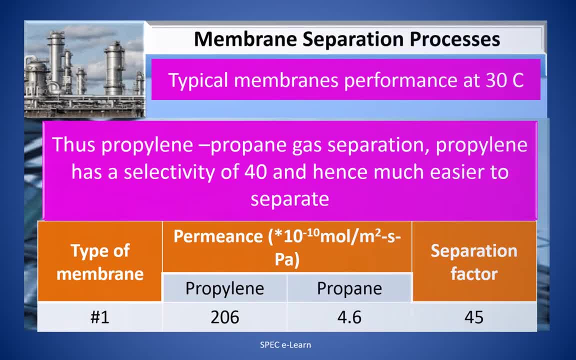 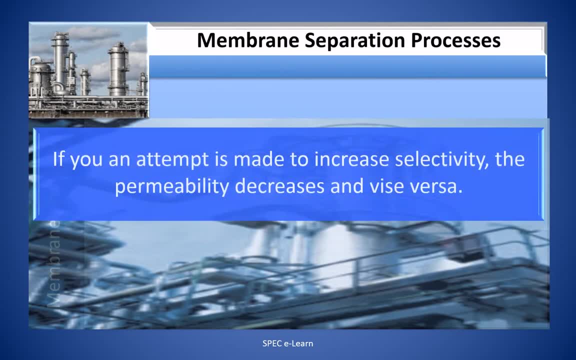 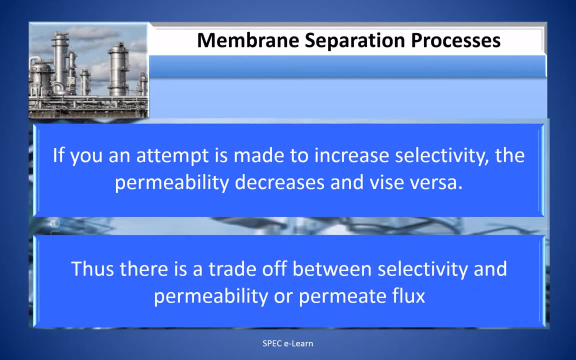 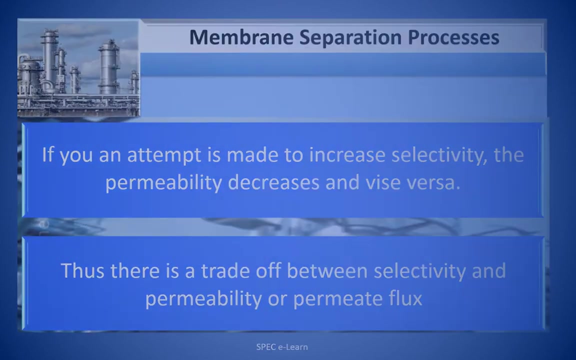 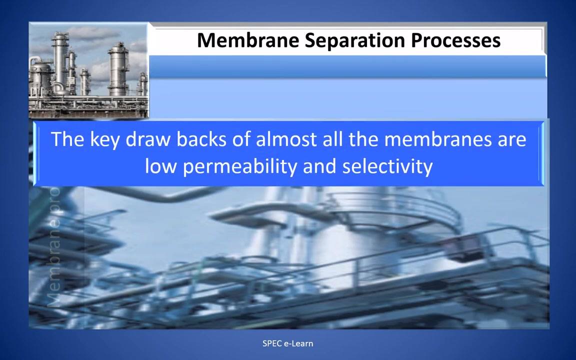 much easier to separate. If an attempt is made to increase the selectivity, the permeability will decrease, and vice versa. Thus there is a trade-off between selectivity and permeability, or permeate flux. The key drawbacks of almost all membranes are 1.. 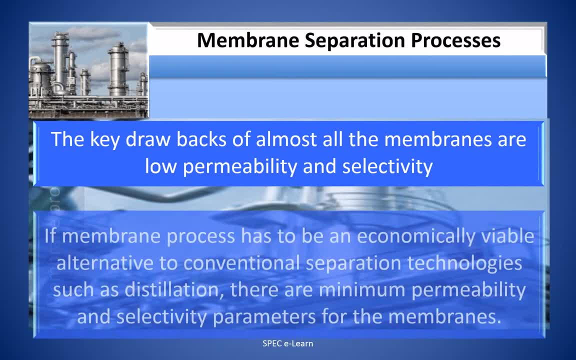 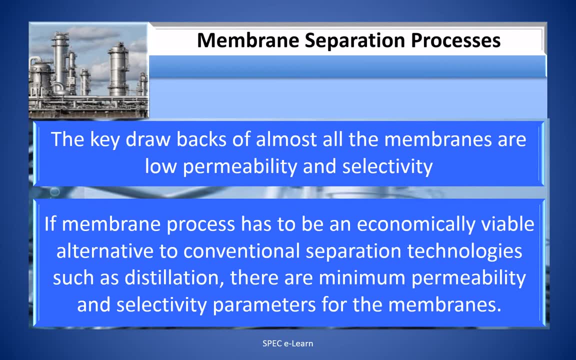 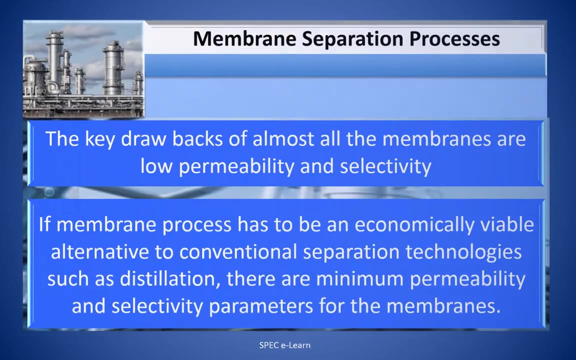 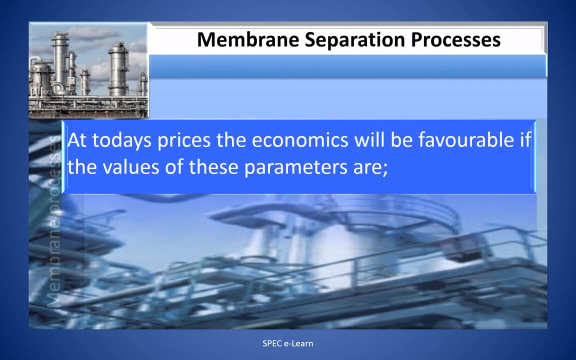 Low permeability and selectivity. If membrane process has to be economically viable alternative to conventional separation technologies such as distillation, there are minimum permeability and selectivity parameters for the membranes. At today's membrane prices, the economics will be favorable if the values of these parameters 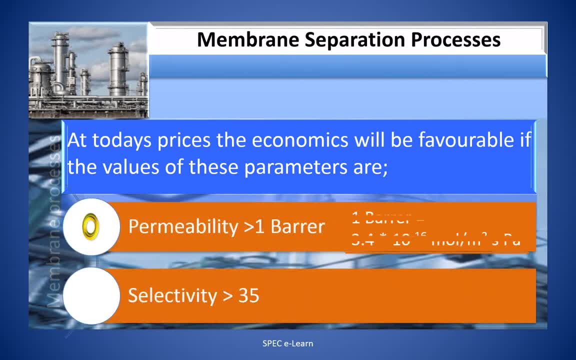 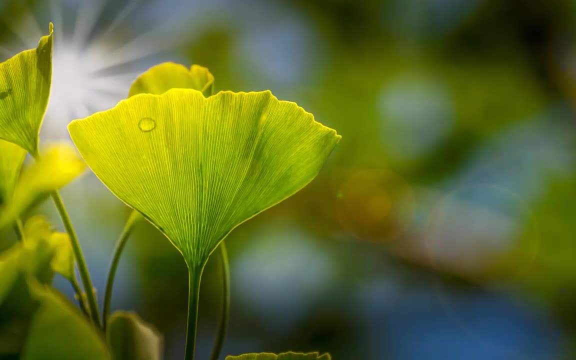 are: 1.. Permeability greater than 1 bar: 1 bar equal to 3.4 times 10 to the power, minus 16 more per square meter. second pascal: Selectivity: greater than 35.. Single stage versus multi-stage membrane system. 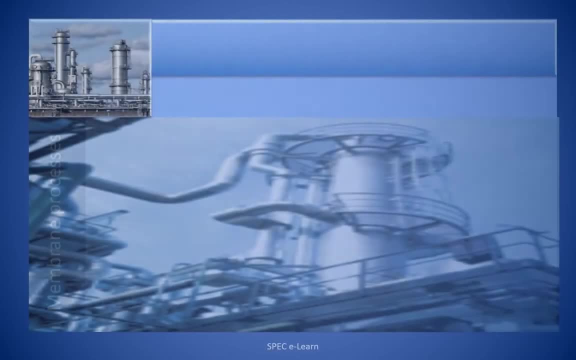 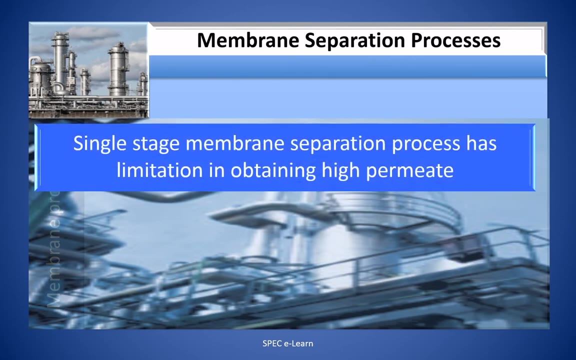 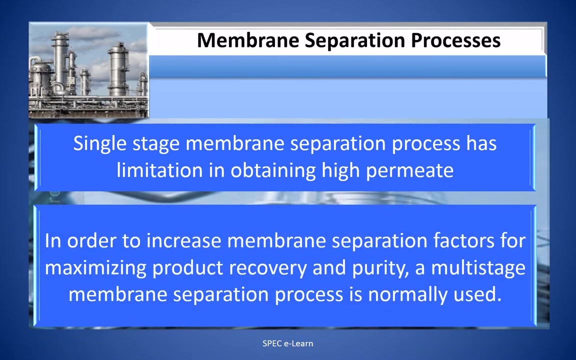 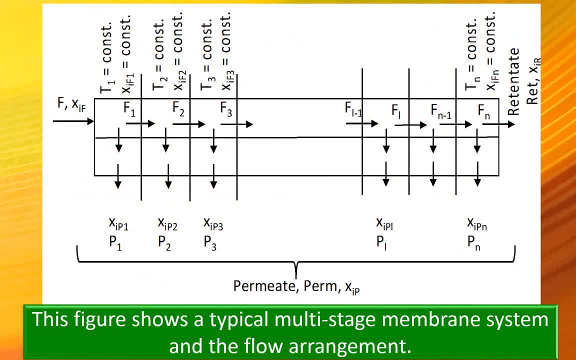 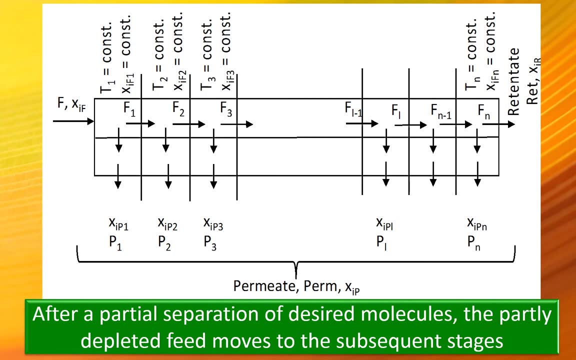 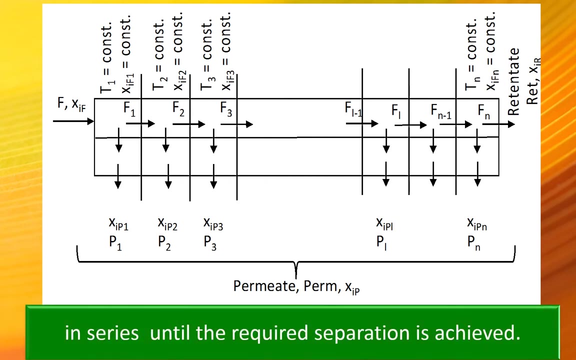 This figure shows a typical multi-stage membrane system and the flow arrangement. It consists of several Cells of membrane connected in series. The feed enters the first stage After a partial separation of desired molecules. the partly depleted feed moves to the subsequent stages in series until the required separation is achieved. 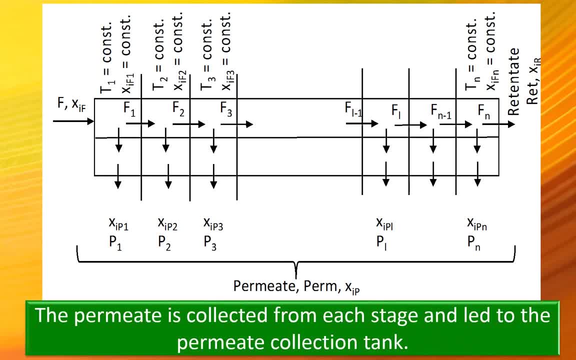 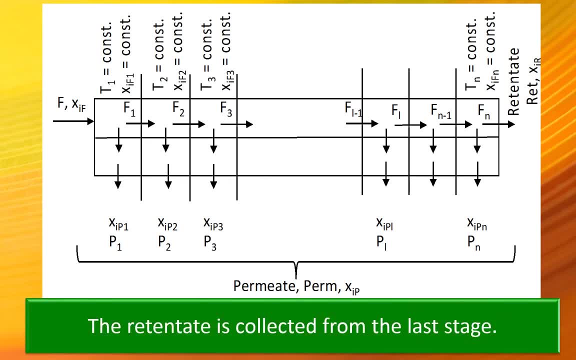 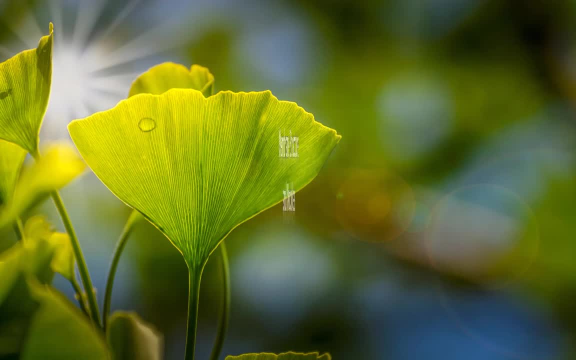 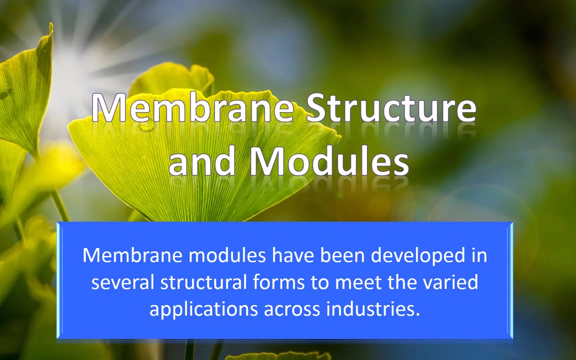 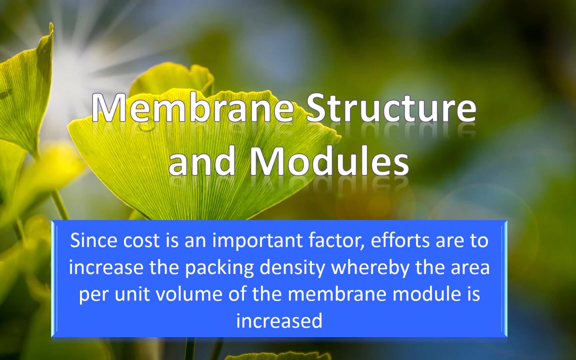 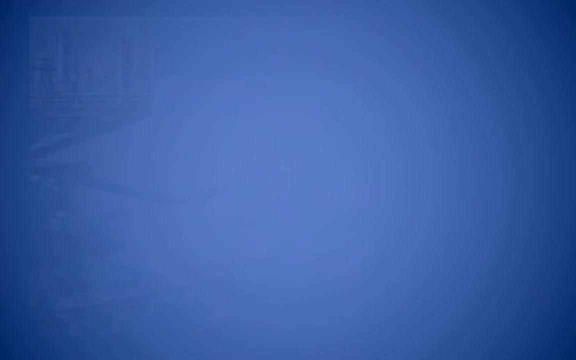 The permeate is collected from each stage and led to the permeate collection tank. The return date is collected from the last stage. The membrane can then be Davy to be resolved via a 96 degree feeding process. The membrane is then transformed into a multi-stage membrane system and then ready to be re-treated. 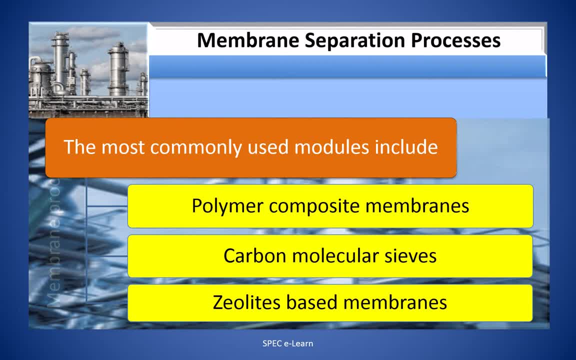 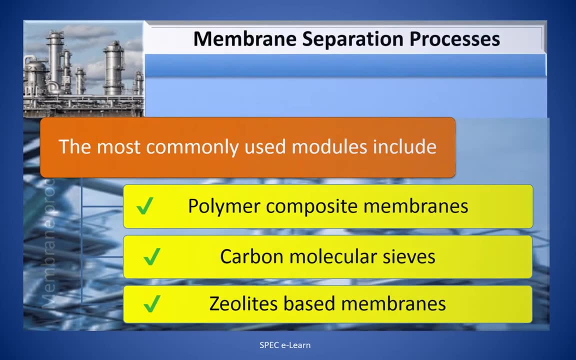 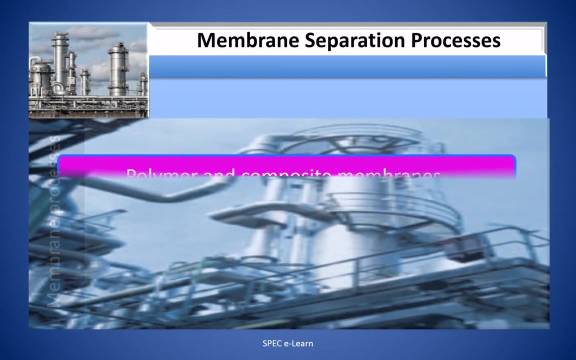 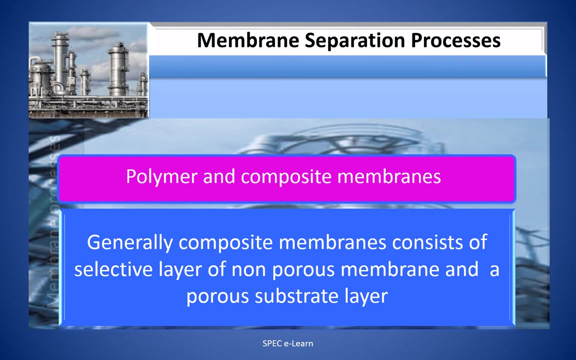 2. Varying of membrane volume. 3. 2. Membranes have been developed out of materials that include polymer, composite membranes, carbon, molecular sieves, zeroed-based membranes, Polymer and Composite Membranes. Generally, composite membrane consists of a selective layer of non-porous membrane and a porous substrate layer. 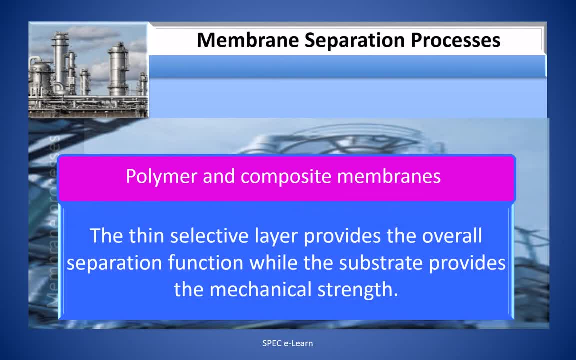 The thin selective layer provides the overall separation function, whereas the substrate layer provides the overall separation function. Whereas the substrate layer provides the overall separation function. A typical example is a GFT PVA composite membrane that comprises PVA selective layer and a PAN supporting layer and a non-woven support layer. 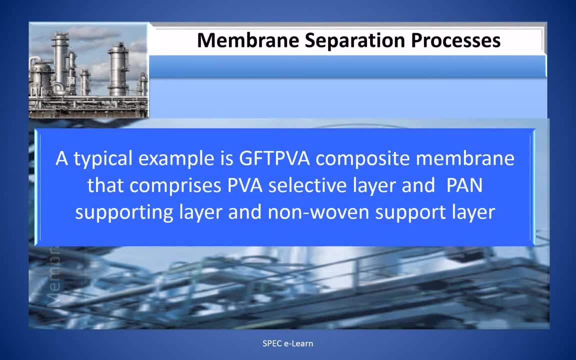 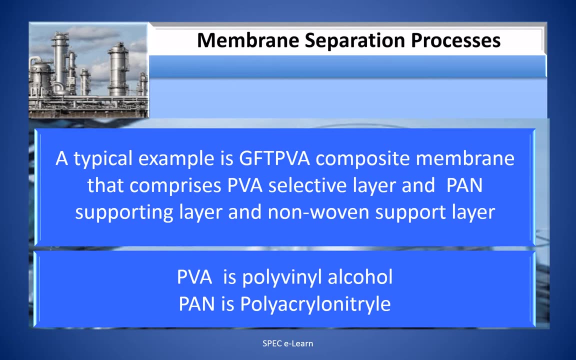 A typical example is a GFT PVA composite membrane that comprises PVA selective layer and a PAN supporting layer and a non-woven support layer. PVA is polyvinyl alcohol, PAN is polyacrylonitrile. This figure illustrates the structure of a composite membrane. 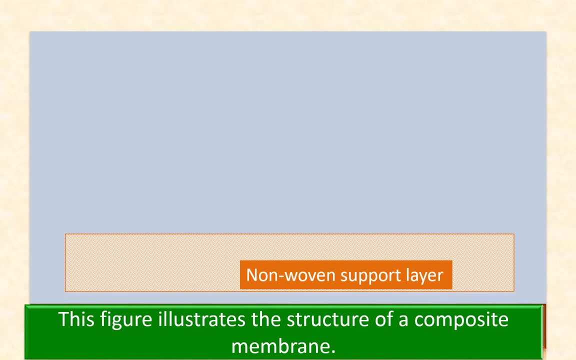 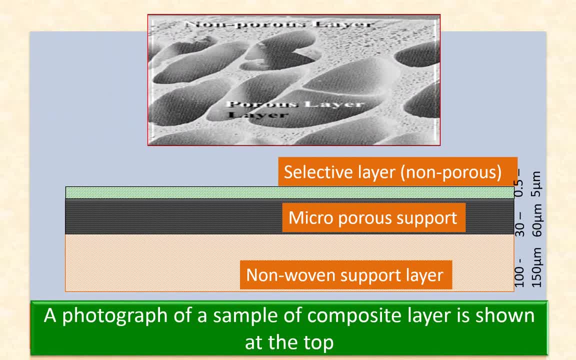 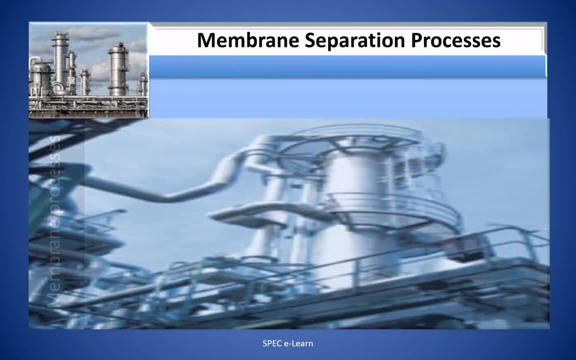 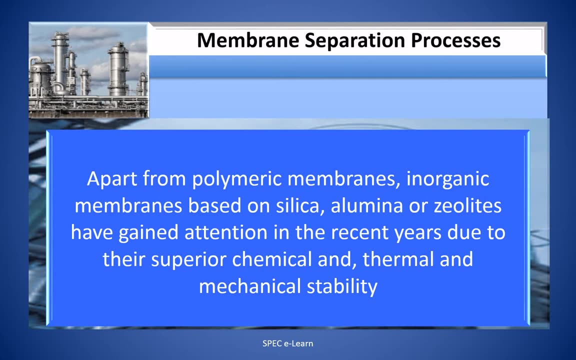 A photograph of a sample of composite layer is shown at the top. A photograph of a sample of composite layer is shown at the top. shown at the top. Apart from the polymeric membranes, inorganic membranes based on silica, alumina or zeolites. 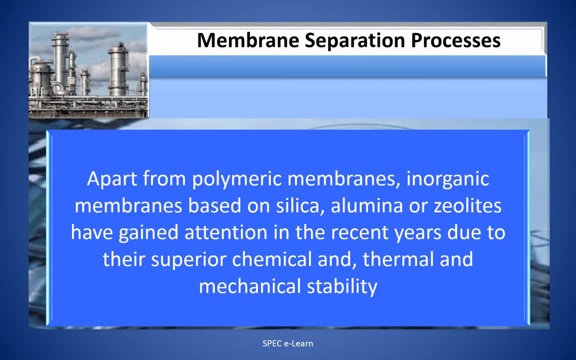 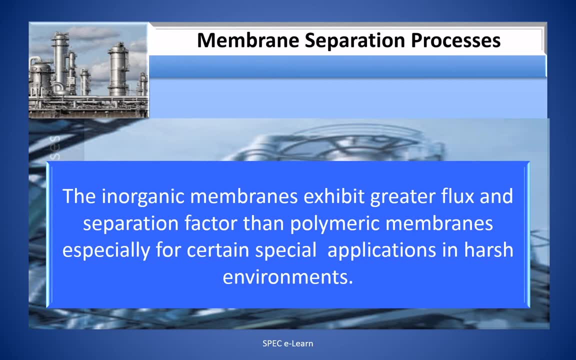 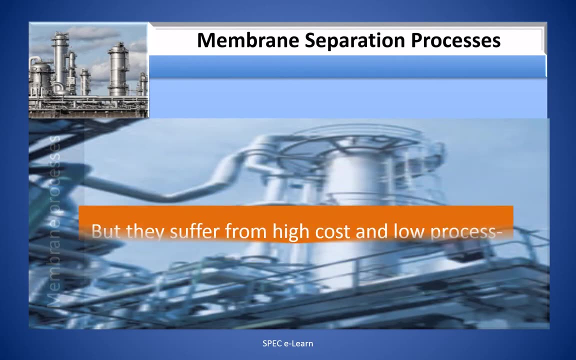 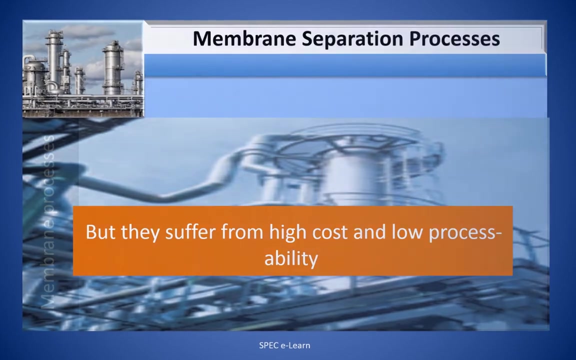 have gained attention in the recent years due to their superior chemical and thermal and mechanical stability. The inorganic membranes exhibit greater flux and separation factor than polymeric membranes, especially for certain special applications in harsh environments, but they suffer from high cost and low processability. 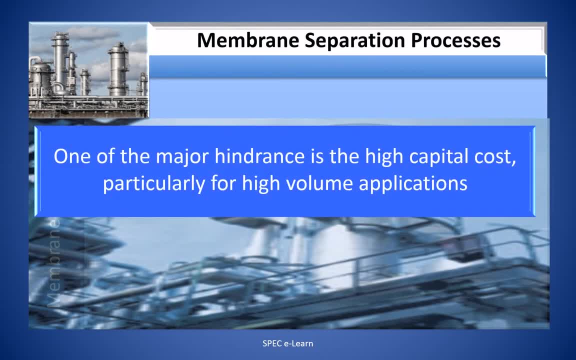 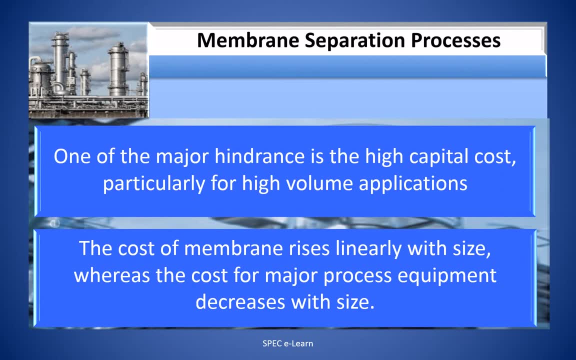 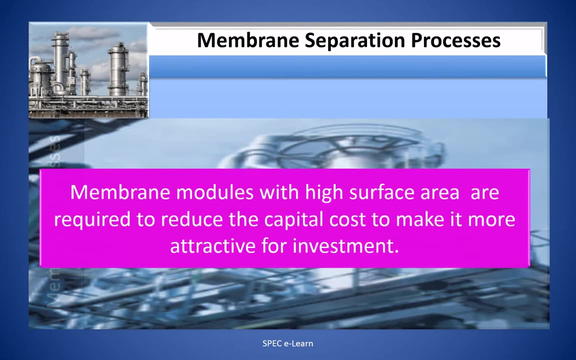 One of the major hindrance is the high capital cost, particularly for high-volume applications. The cost of membrane rises linearly with size, whereas the cost for major process equipment decreases with size. Membrane modules with high surface area are required to reduce the capital cost to make. 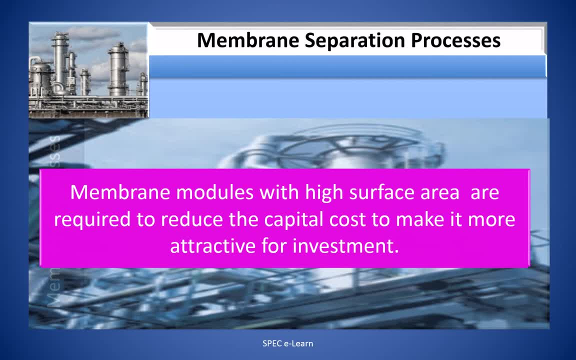 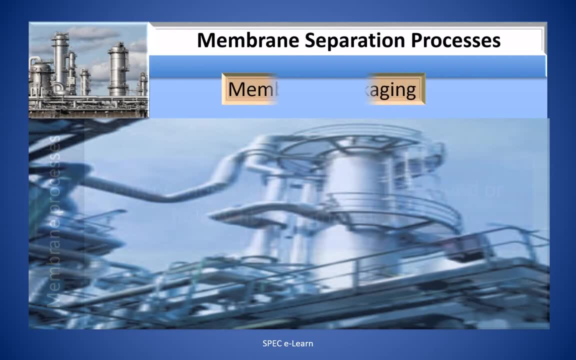 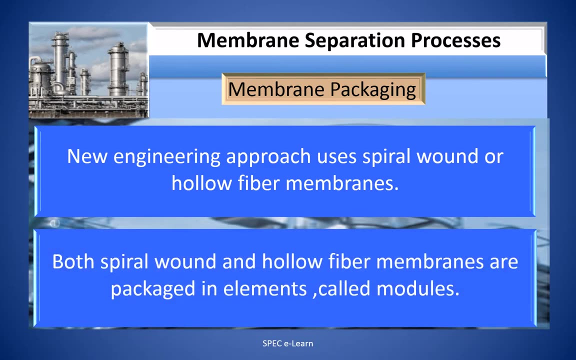 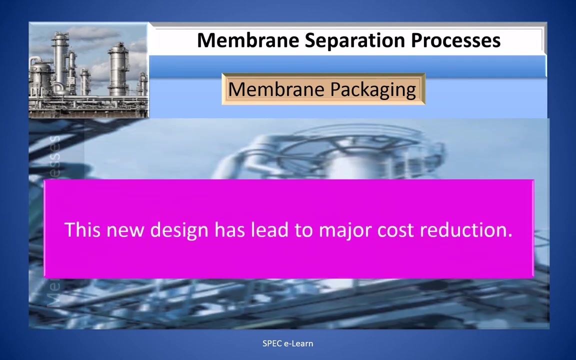 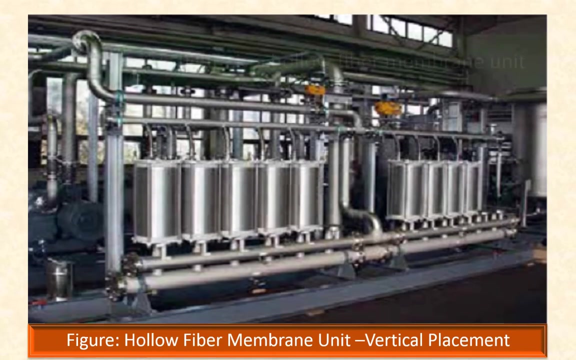 it more attractive for investment. New engineering approach uses spiral-bound or hollow-fibre membranes. Both spiral-bound and hollow-fibre membranes are packaged in elements called modules. This new design has led to major cost reduction. Shown in this figure is a hollow-fibre membrane unit. 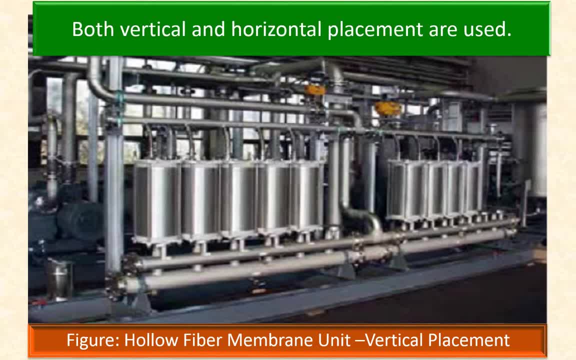 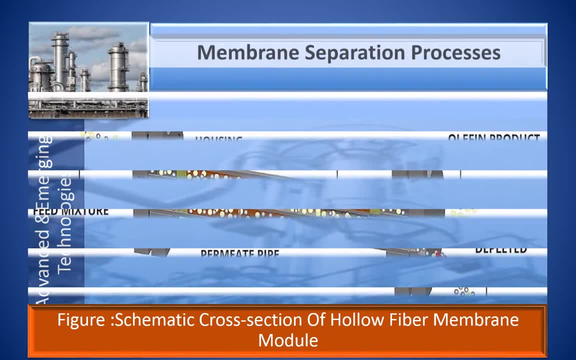 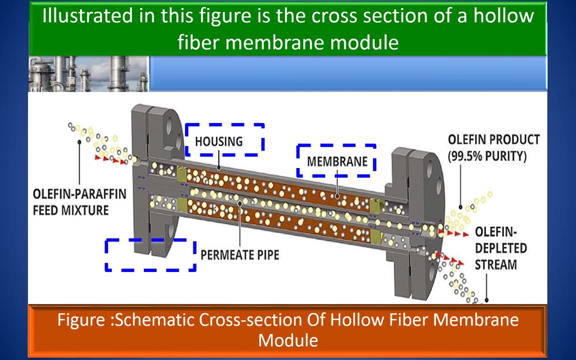 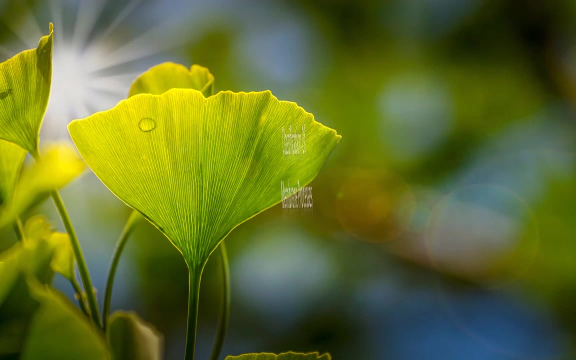 Both vertical and horizontal placements are used. Illustrated in this figure is the cross-section of a hollow-fibre membrane. The membrane is enclosed in the housing. The permeate is collected in the central pipe, as shown. Observe the feed, The permeate and the retentate streams movement through the hollow-fibre unit. 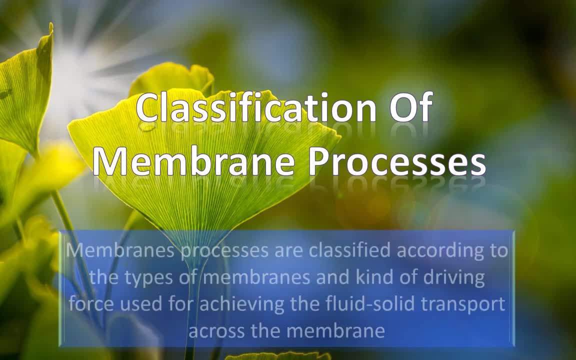 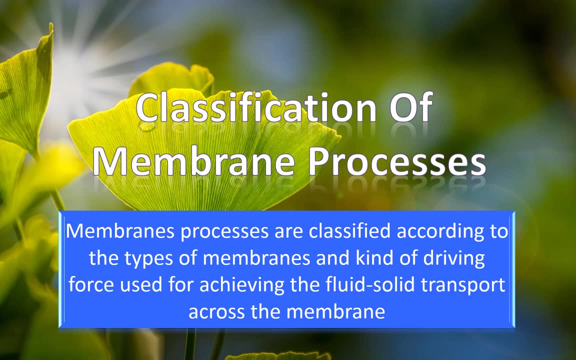 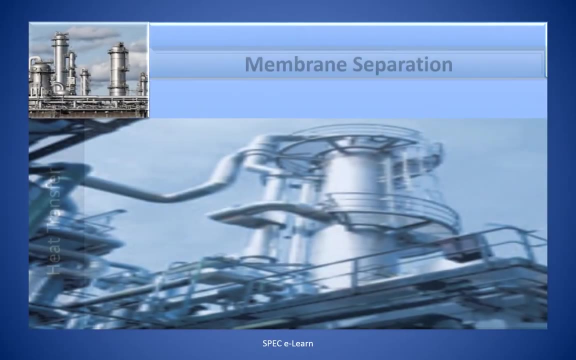 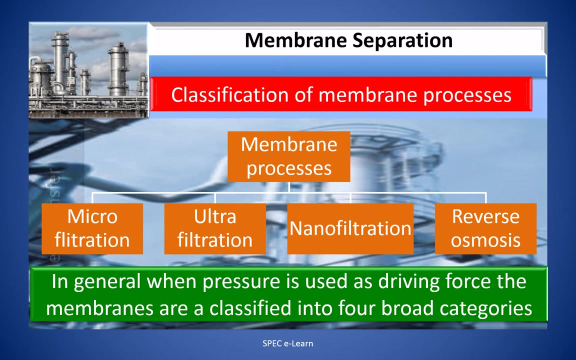 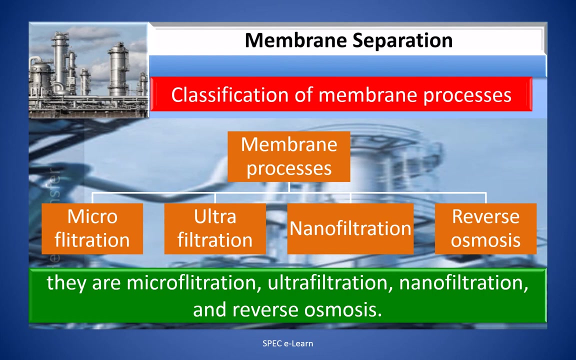 Classification of Membrane Processes. Membrane processes are classified according to the types of membrane, Such as the general flow, the main lines and the D- runs of the membrane, the fluids into the membrane. Other membrane processes that has emerged recently are per-operation and gas separation. 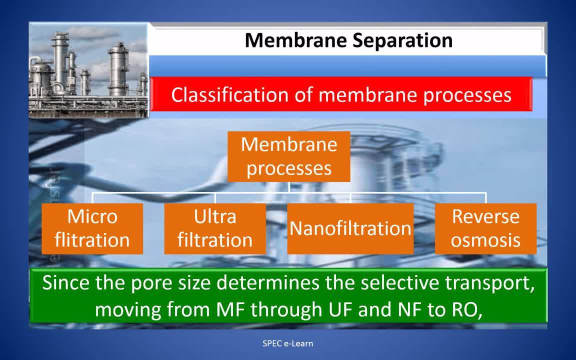 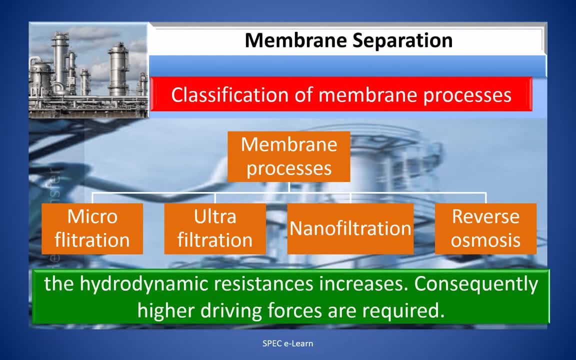 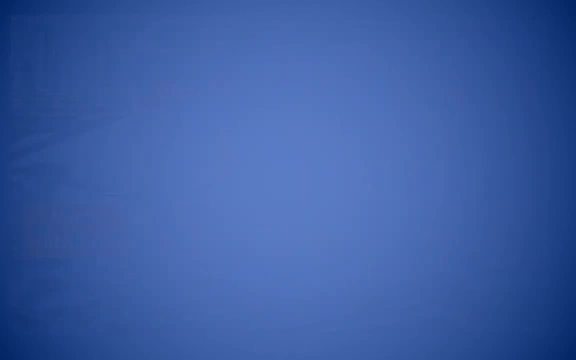 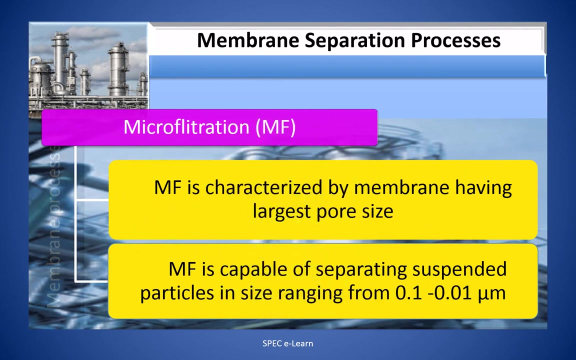 Since the pore size determines the selective transport moving from MF through UF and NF to RO, the hydrodynamic resistance increases. Consequently, higher driving forces are required. Microfiltration: Microfiltration is characterized by membrane having large pore size. It is capable of separating suspended particles in sizes ranging from 0.1 to 0.01 micrometer. 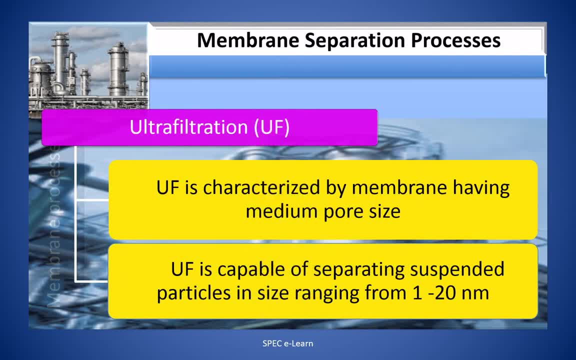 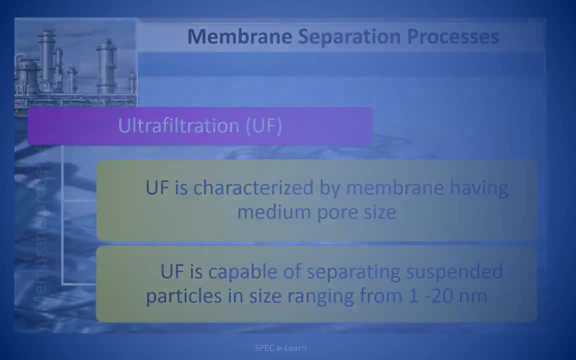 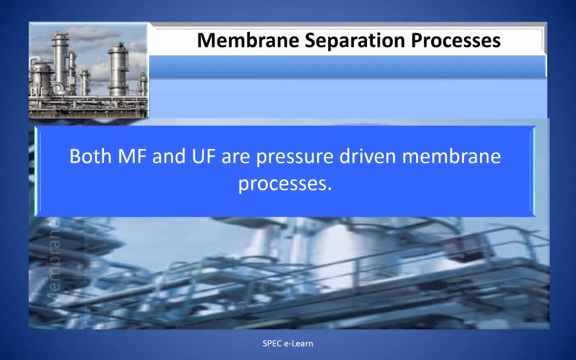 UF is capable of separating suspended particles in sizes ranging from 1 to 20 nanometers. Both microfiltration and ultrafiltration are pressure-driven membrane processes. The sieving effects are such that the membrane is a thin film which can be separation of allowable particles for engineering purposes. 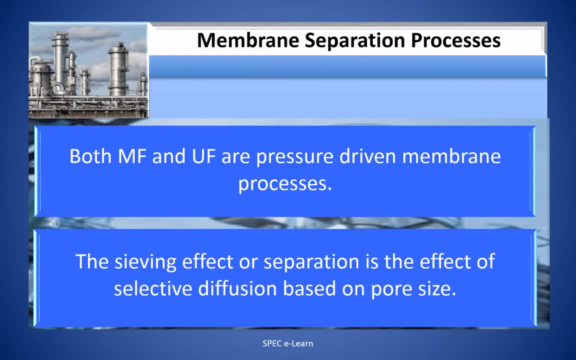 MF is self-continuous and ile Achofully broken by a medium pore-sized membrane. The microfiltration is characterized by membrane having medium pore size. UF is capable of separating suspended particles in sizes ranging from 1 to 20 nanometers. separation is the effect of selective diffusion based on pore size. 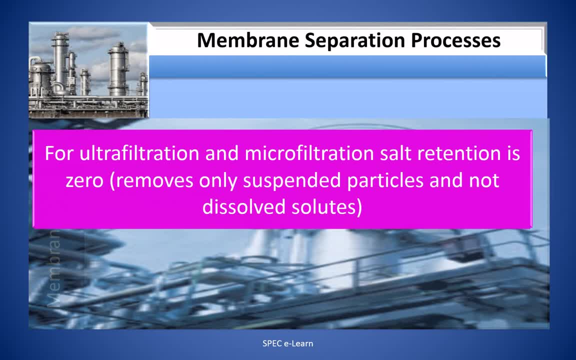 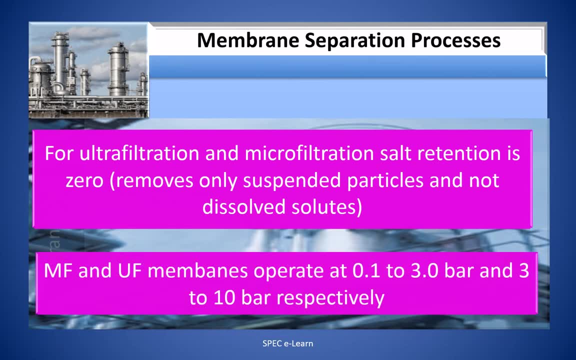 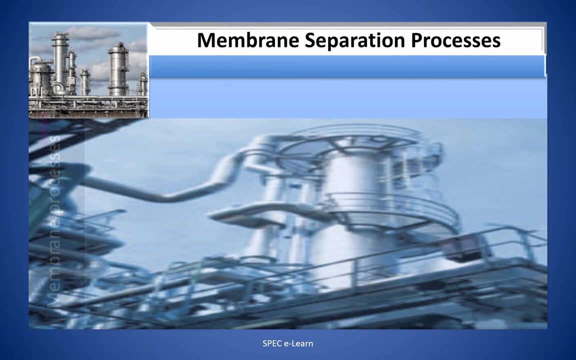 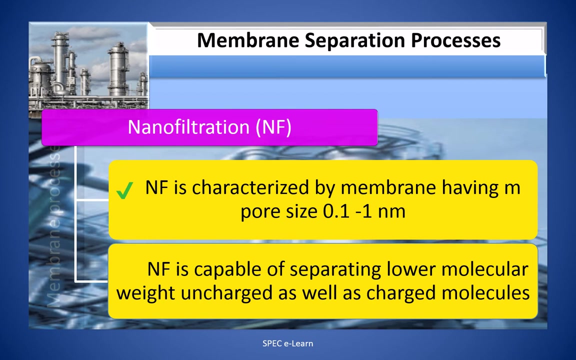 For ultrafiltration and microfiltration, salt retention is zero, ie it removes only suspended particles and not dissolved solutes. MF and UF membranes operate at 0.1 to 3 bar and 3 to 10 bar respectively. Nanofiltration is characterized by membrane having pore size varying from 0.1 to 1 nm. 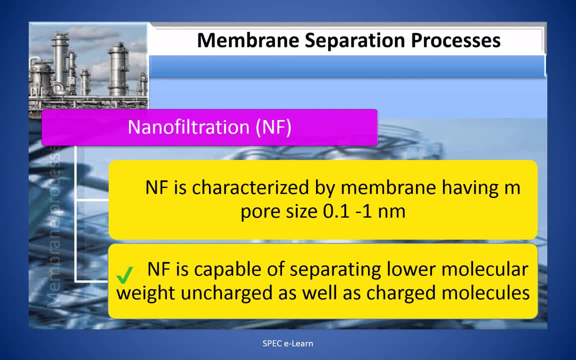 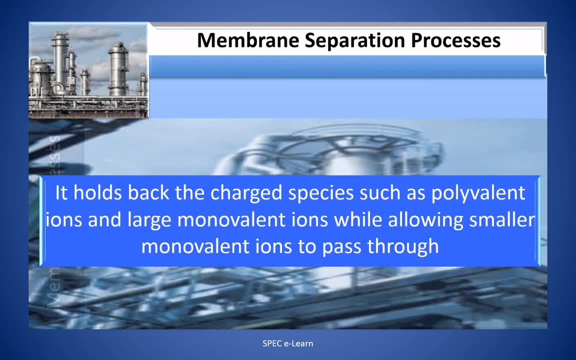 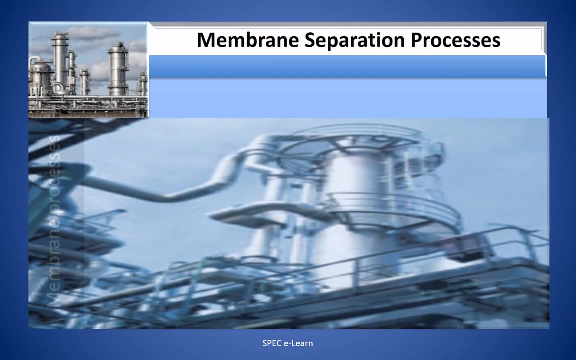 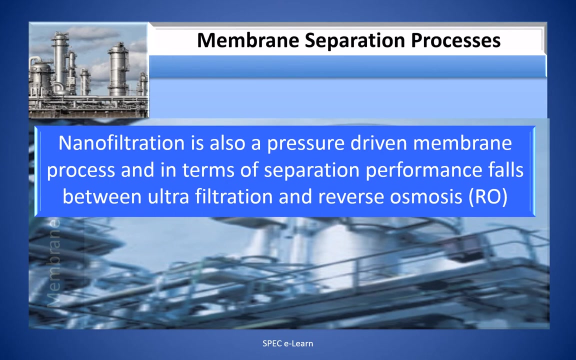 NF is capable of separating lower molecular weight, uncharged as well as charged molecules. It holds back the charged species, such as polyvalent ions and large monovalent ions, while allowing smaller monovalent ions to pass through. Nanofiltration is a pressure-driven membrane process and in terms of separation performance. 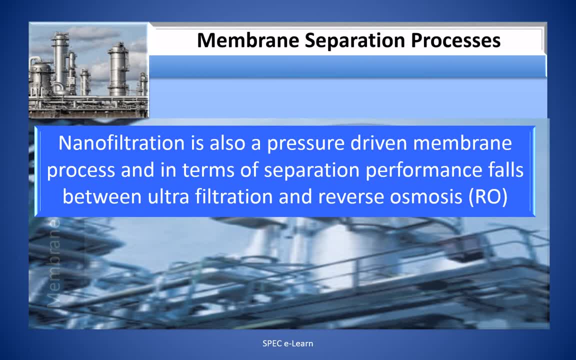 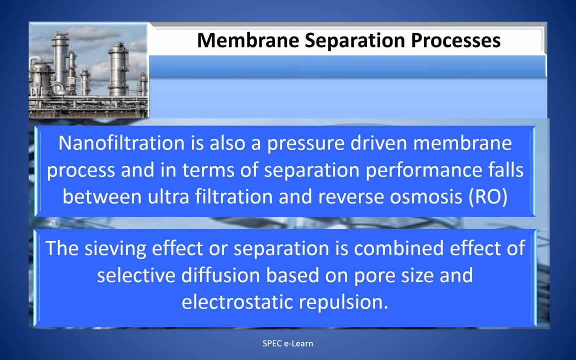 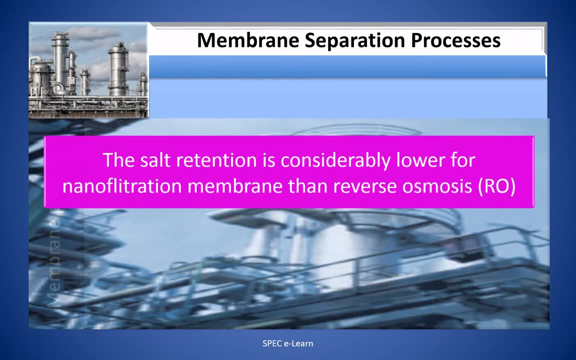 falls between ultrafiltration and reverse osmosis. The sieving effect of separation is combined effect of selective diffusion based on pore size and electrostatic repulsion. The salt retention is considerably lower. For nanofiltration The operating pressure is in the range of 20 to 30 bar. 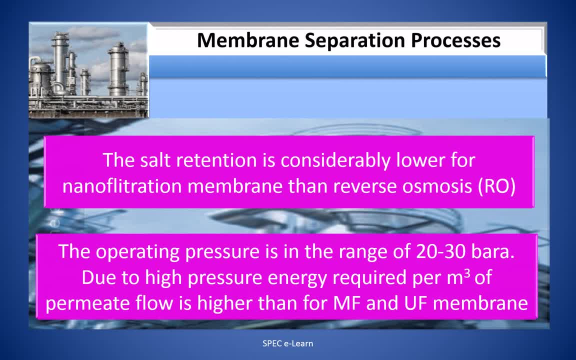 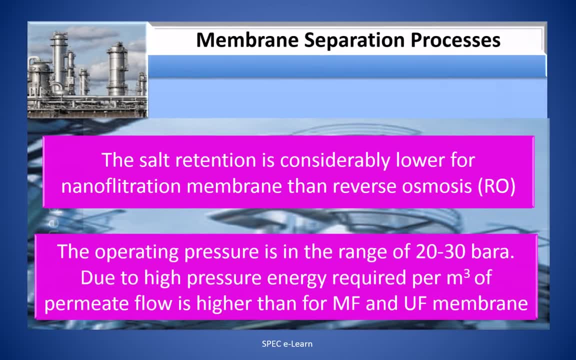 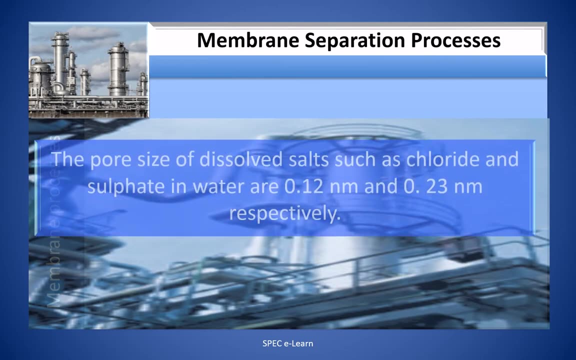 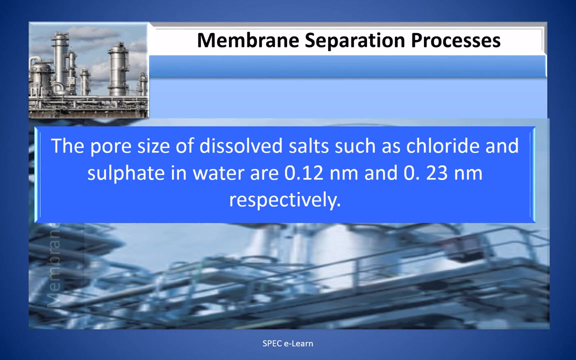 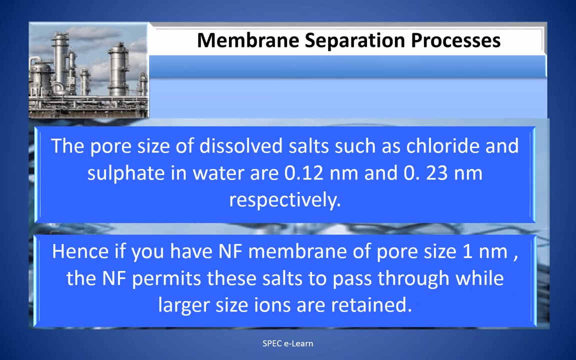 Due to high pressure, energy required per meter cube of permeate flow is higher than for MF and UF membranes. The pore size of dissolved salts such as chloride and sulphate in water, or 0.1 to 3 bar, is higher. Hence, if you have a nanofiltration membrane of pore size 1 nm, the NF permits these salts. 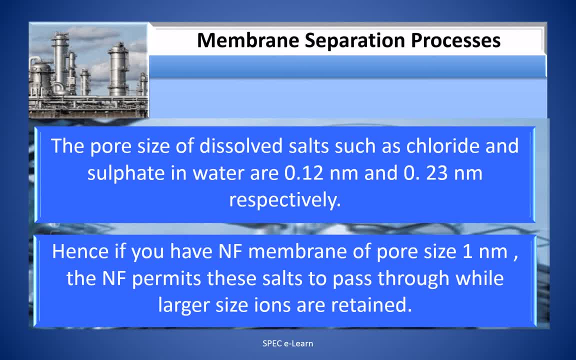 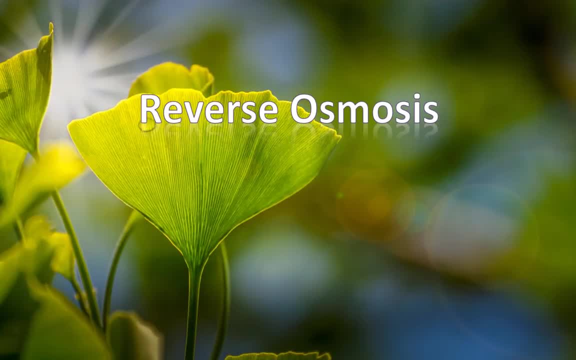 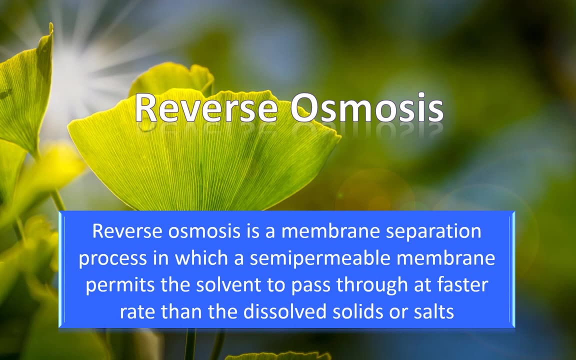 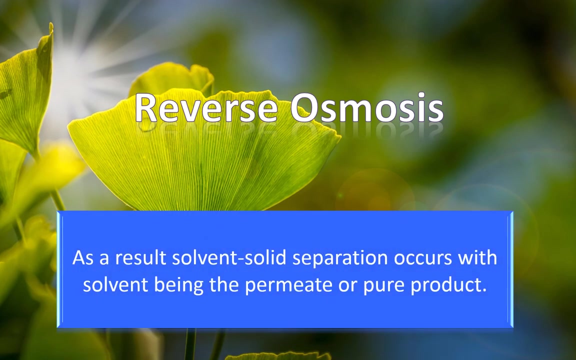 to pass through, while larger size ions are retained. Reverse osmosis is the membrane separation process in which a semipermeable membrane permits solvent to pass through. The solvent to pass through at a faster rate than the dissolved solids or salts. As a result, the solvent-solid separation occurs, with solvent being the permeate or 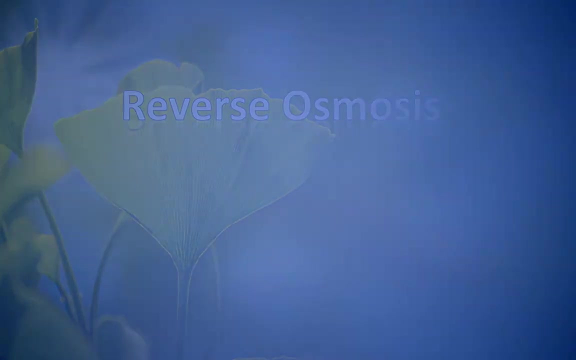 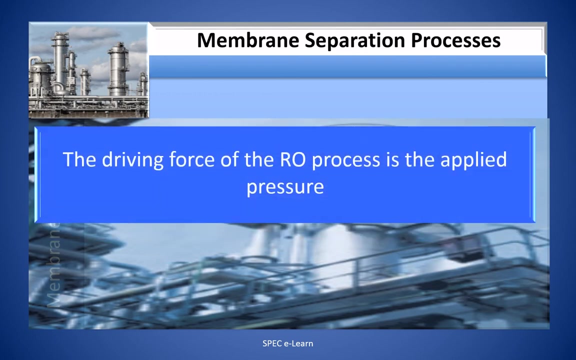 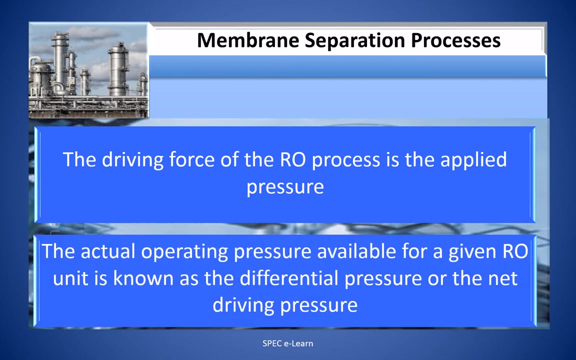 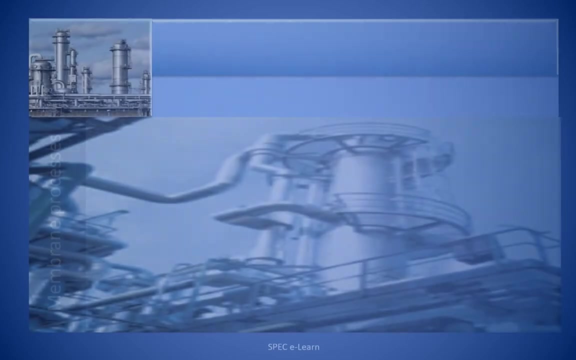 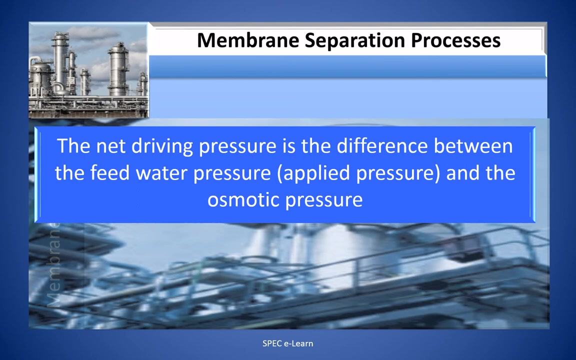 pure product. The driving force of the RO process is the applied pressure. The actual operating pressure available for a given RO unit is known as the differential pressure or the net driving pressure. The net driving pressure is a difference between the feed water pressure or applied pressure. 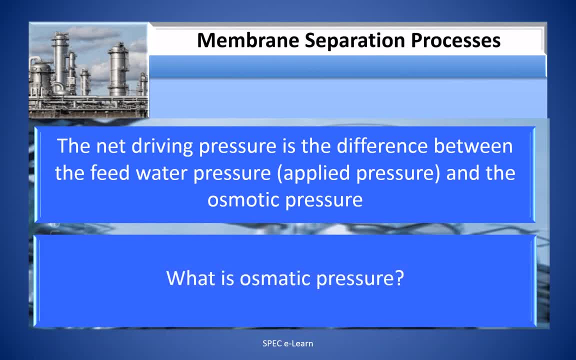 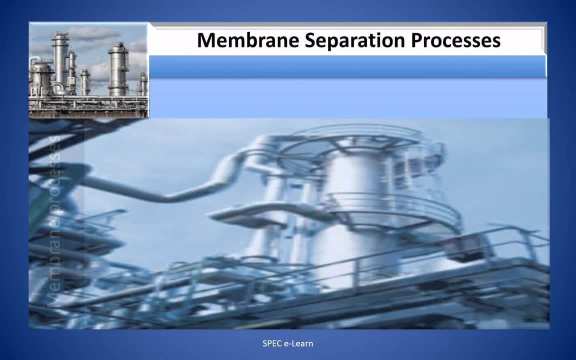 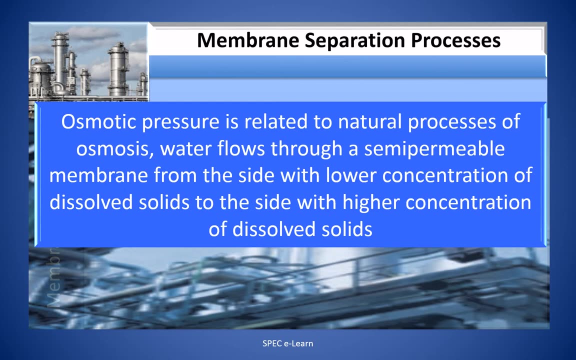 and the osmotic pressure. What is osmotic pressure For the osmotic pressure loss laboratory test? Water is related to the natural process of osmosis. Water flows through a semipermeable membrane from the side with lower concentration of. 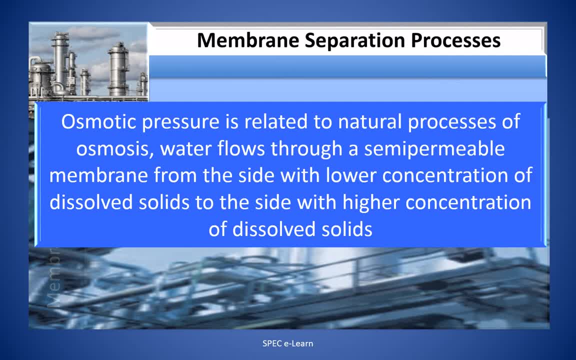 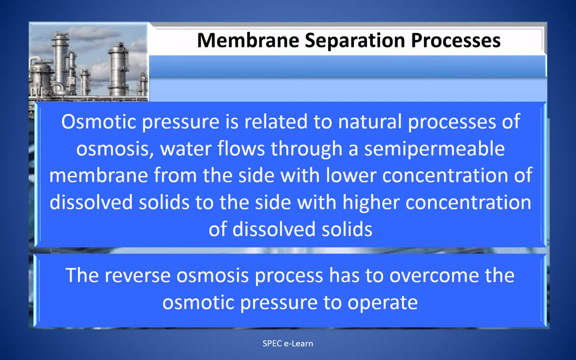 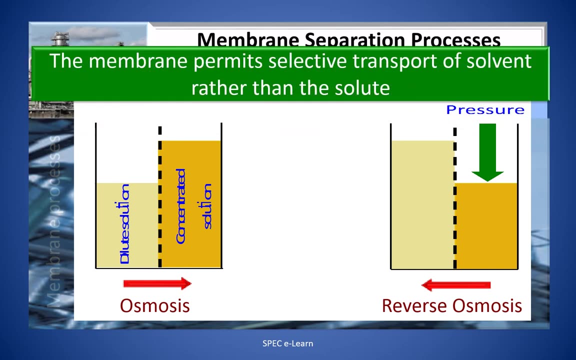 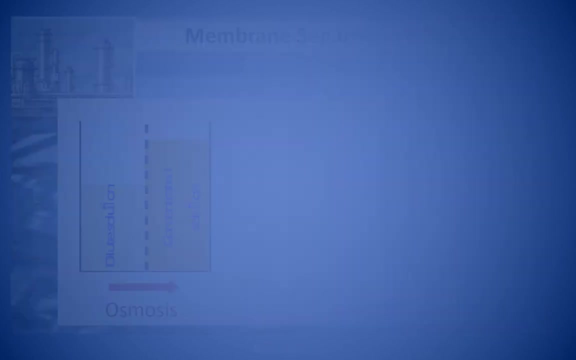 dissolved solids to the side. with higher concentration of dissolved solids, The reverse osmosis process has to overcome the osmotic pressure. to operate, The pressure is applied to overcome the osmotic pressure. The membrane permits a selective transport of solvent rather than the solute. 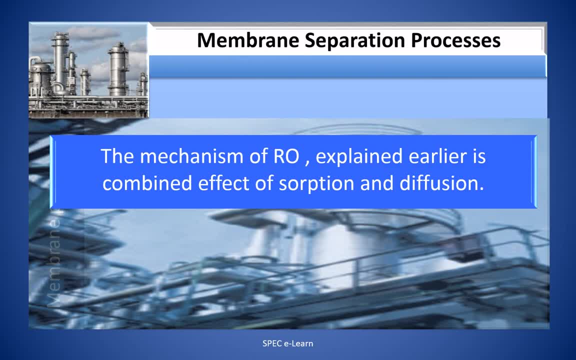 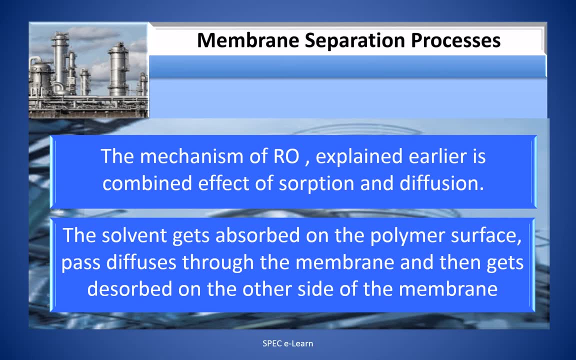 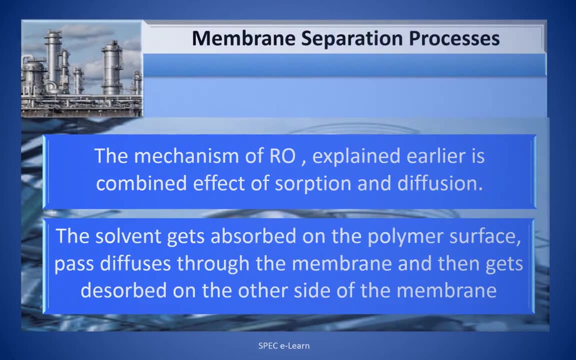 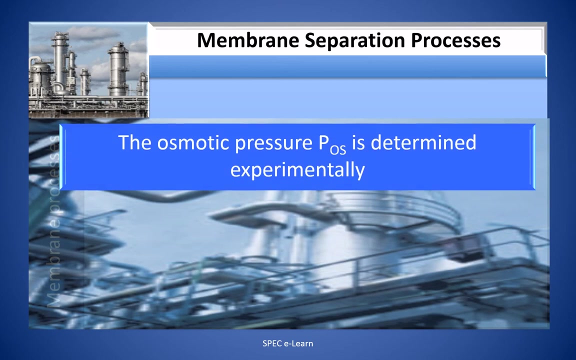 The mechanism of RO, as explained earlier, is a combined effect of sorption and diffusion. The solvent gets absorbed on the polymer surface, passes through the membrane and then get desorbed on the other side of the membrane. The osmotic pressure, POS, is determined experimentally. 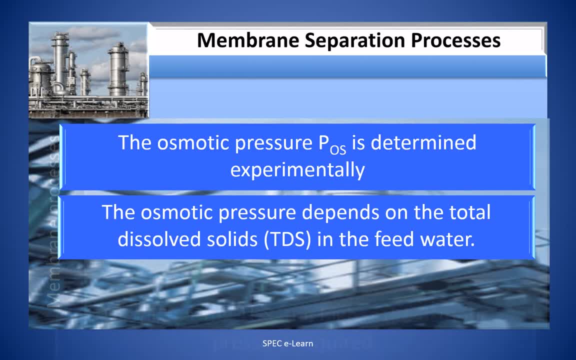 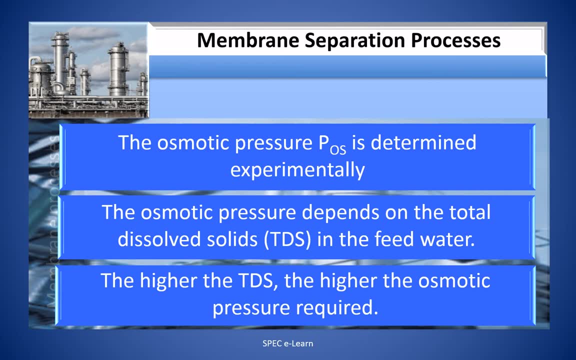 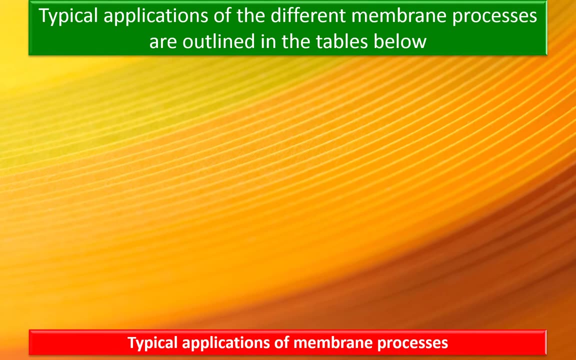 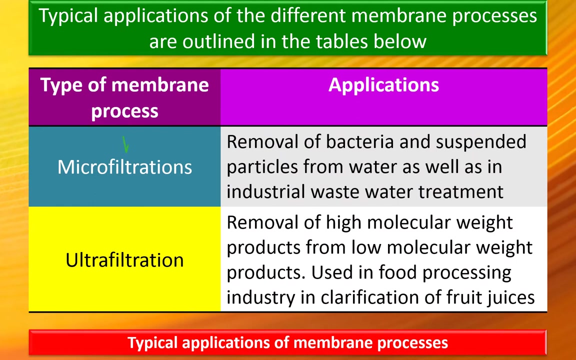 The osmotic pressure depends on the total dissolved solids TDS in the feed water. The higher the TDS, the higher the osmotic pressure required. Typical applications of the different membrane processes are outlined in the table below. Type of Membrane Process: Microfiltration.